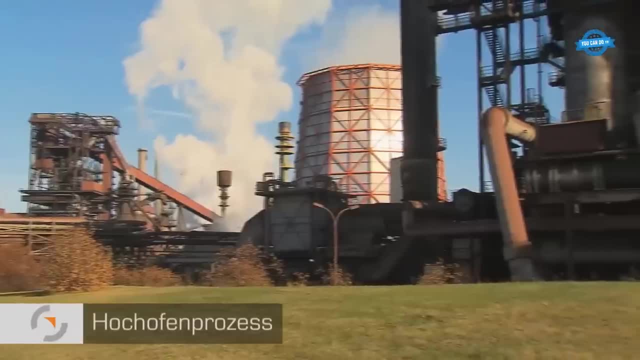 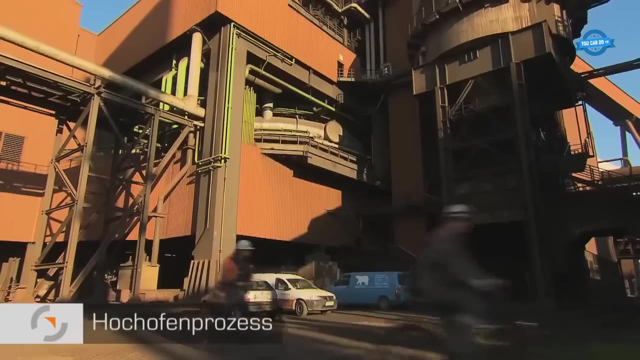 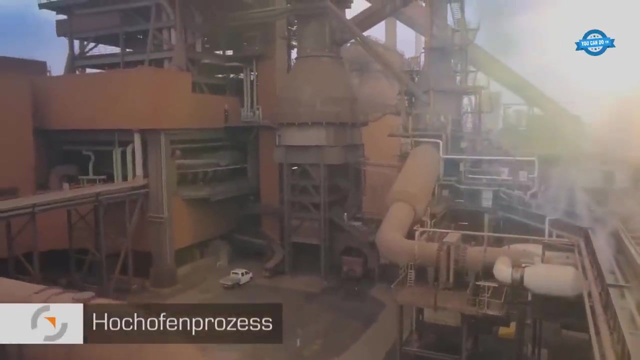 The raw material is processed into fine ore pellets, which are made of iron ore concentrate that is too small to store and transport well, The Salzgitter location has several blast furnaces, with the largest being over 50 meters high. Here up to 14,000 tons of pig iron are produced daily. 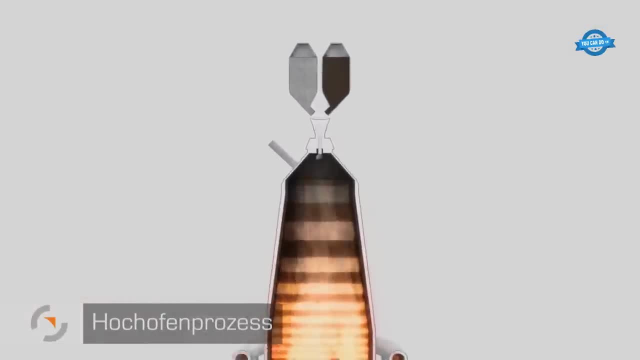 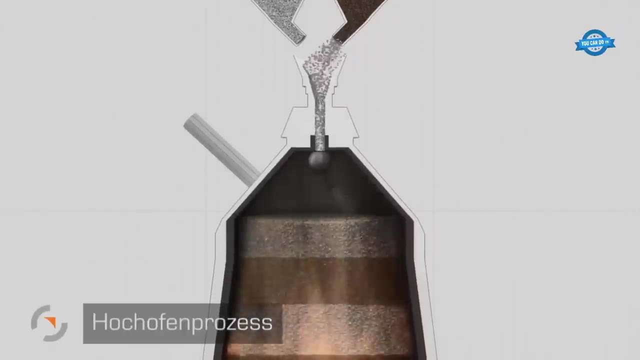 Steel is a precious metal and metalware One of the most important elements for production. Steel is a plastic material. The steel is designed to protect its muye and the surface of the metal, which are obtained by steel. It is a chemical-based metal and it is said that steel is a very high-tech material, so that it is good for all guys and girls. 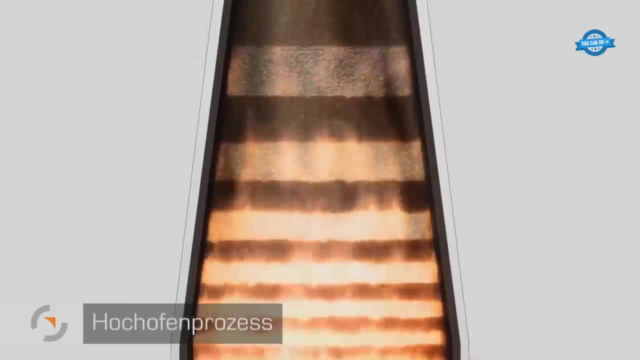 Steel is a high-tech and high-tech material. It is very high-tech material and it is often used for Loading Soap and other things. It is a high-tech material with high weapons and a high-tech material that is easy to fire. 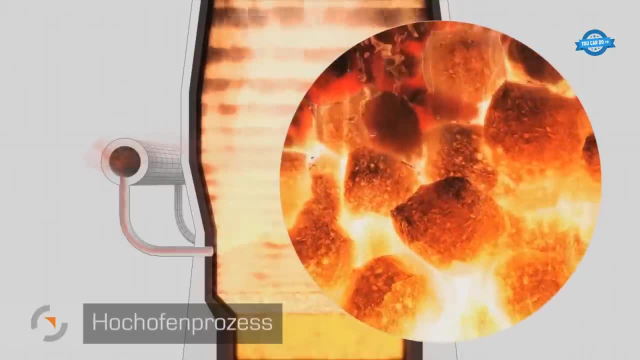 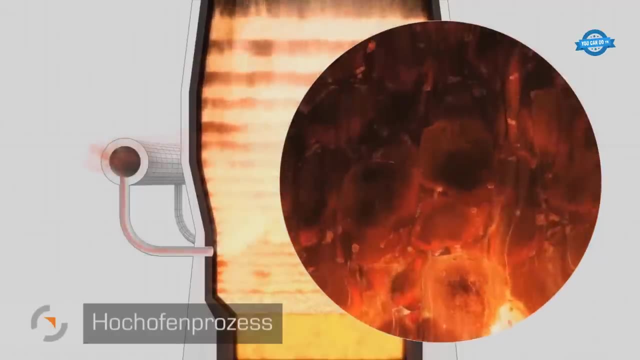 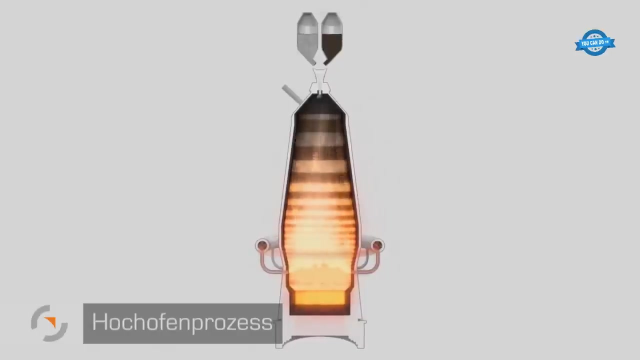 The steel is made of stainless steel. The pig iron is created inside the blast furnace with coke and a layer of heart being alternately given to the furnace shaft. The layers fall down and the ore is heated, reduced and finally melted as it goes through. 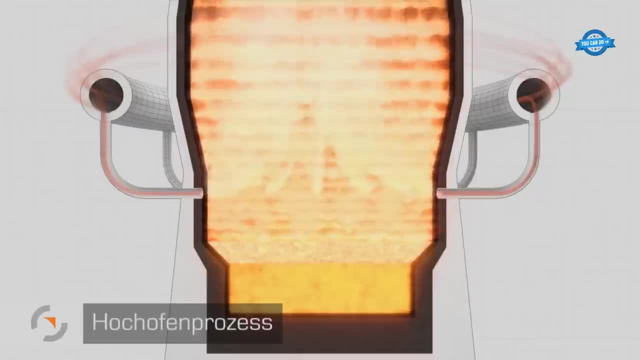 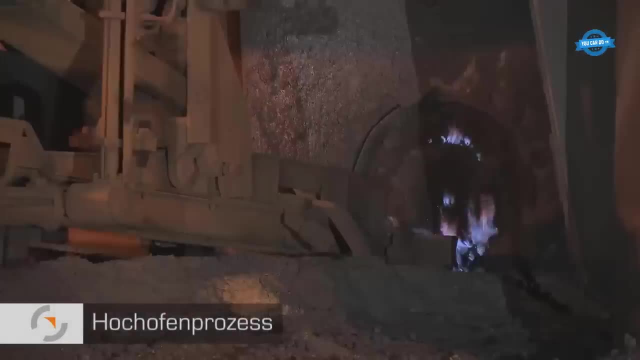 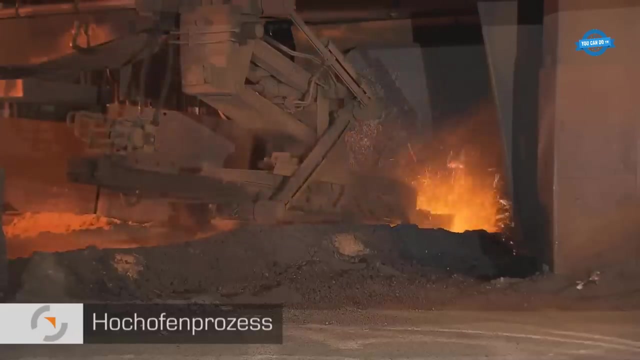 the ascending process gas. The process gas is created by blowing preheated air into the furnace and it burns with the coke product, generating approximately 2,000 degrees Celsius hot process gas. The oxygen from the iron oxide is extracted from the process gas and the heat will show. 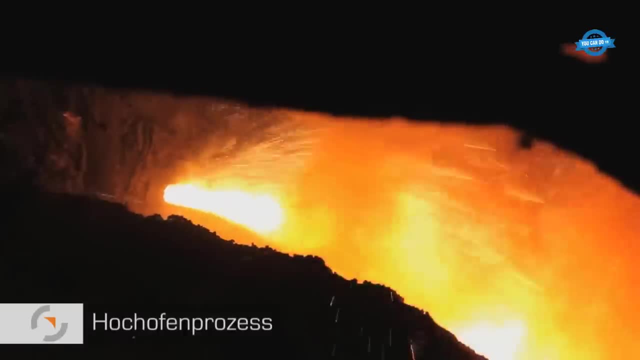 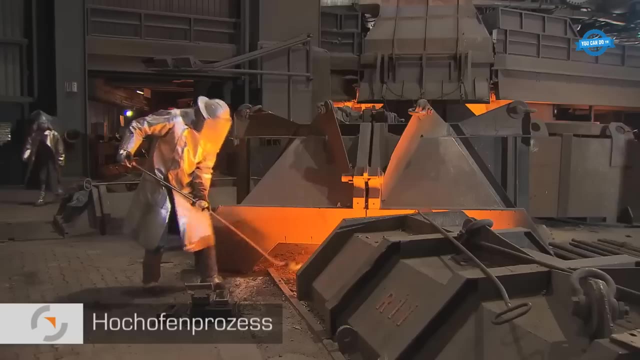 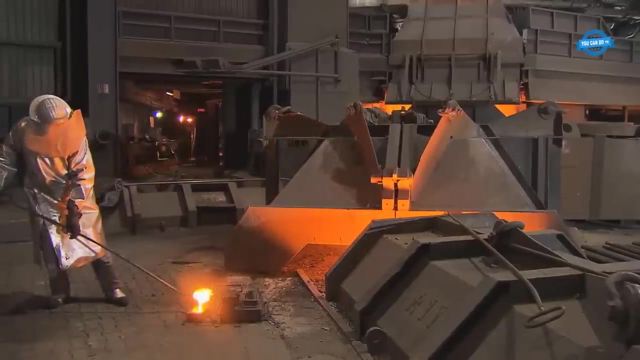 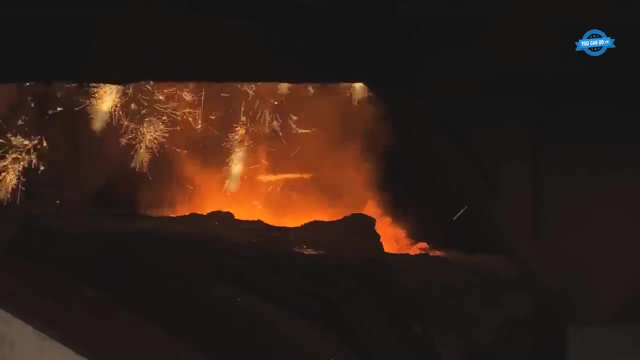 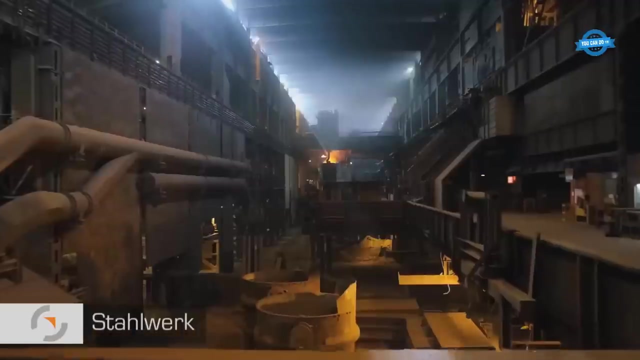 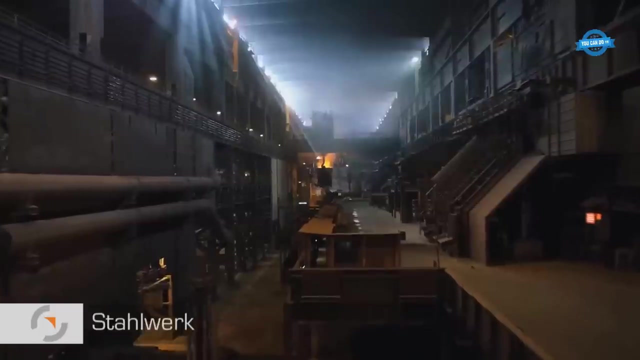 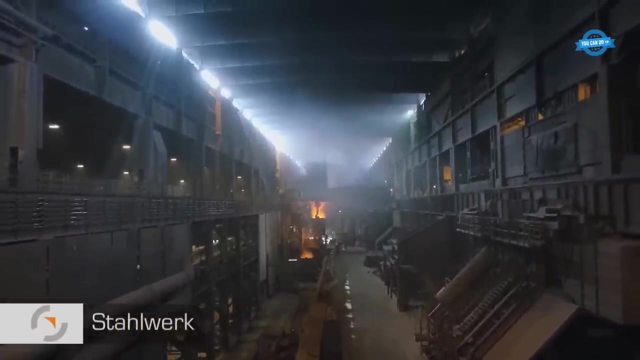 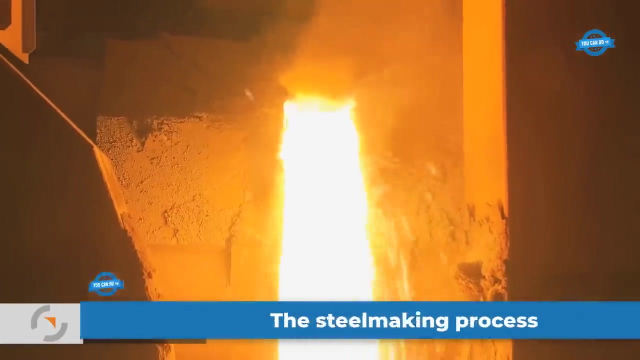 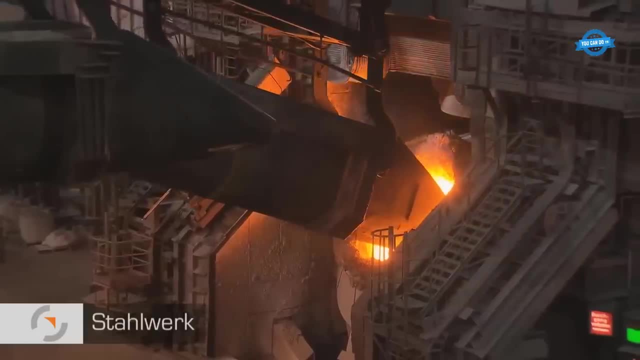 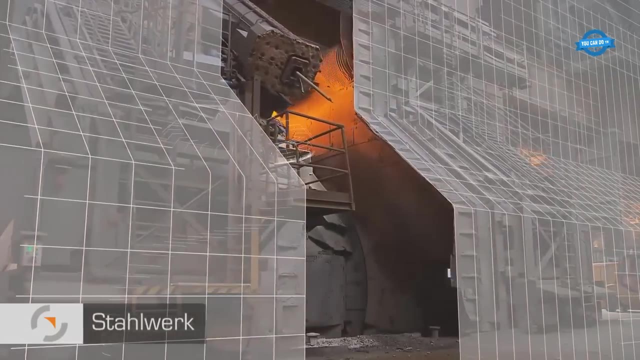 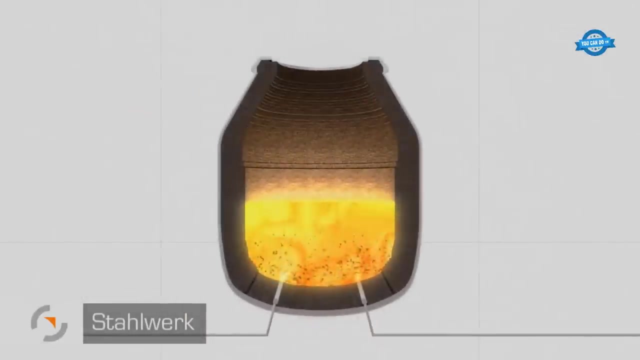 materials. This process takes around 40 minutes, and the resulting raw steel is then sent to the VPL plant for further treatment. At the VPL plant, the crude steel undergoes further processing and refining to achieve the desired chemical composition and mechanical properties. This includes the addition of elements. 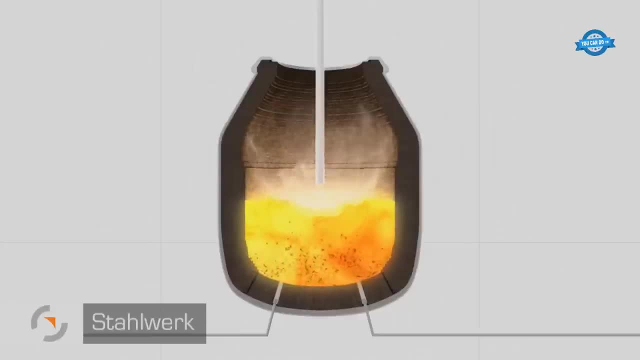 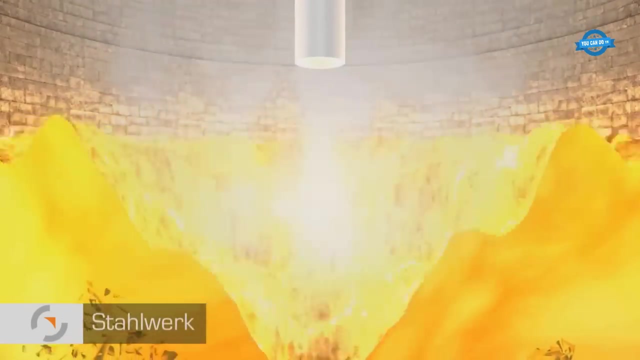 such as manganese, silicon, carbide and molybdenum, to produce steel with individual and high-quality characteristics. The VPL plant uses vacuum ladle alloying technology, which involves the use of a vacuum chamber to prevent the steel from reacting with air during the alloying. 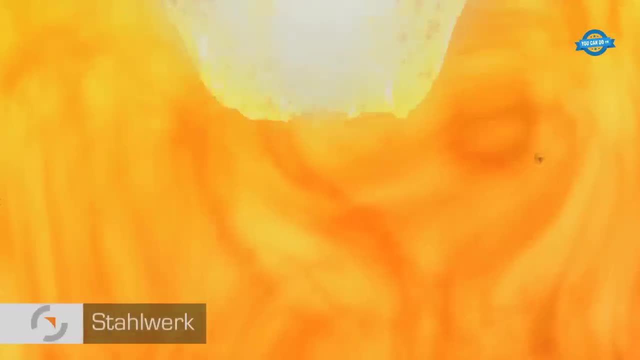 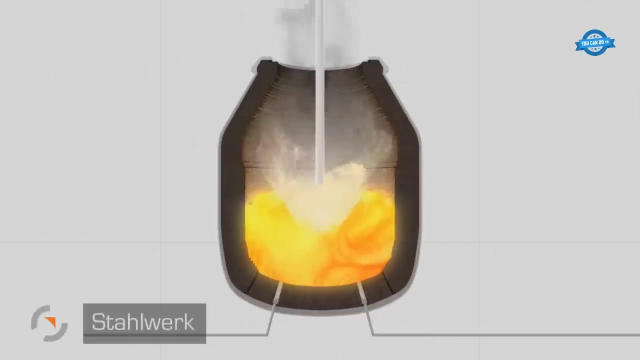 process. This results in the production of high quality and clean steel that is free from impurities and defects. Once the steel has been treated and refined to meet the required specifications, the VPL plant is ready to be used. in the process, Besides the steam running through the steel, it is sent to various rolling 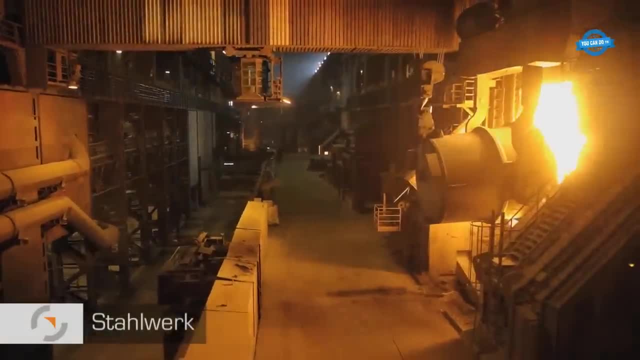 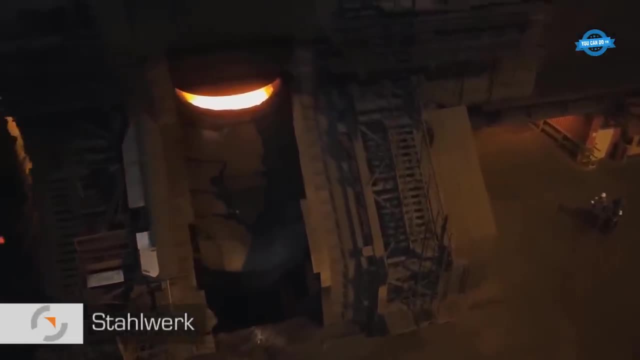 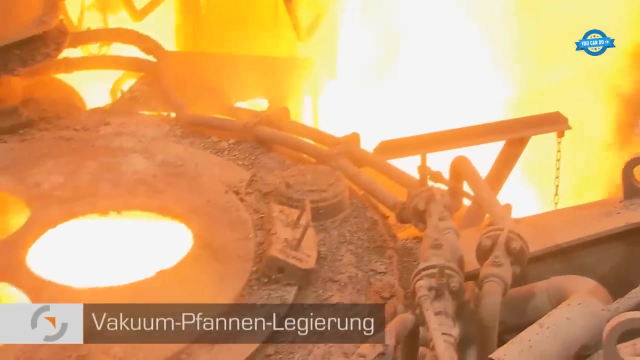 mills for shaping and forming. This includes the hot rolling mill and hot strip line, which use high temperatures and pressure to shape the steel into flat sheets and coils. After the steel is converted into raw steel through the LG converters, it is then transported to the VLA plant, where it is treated in a 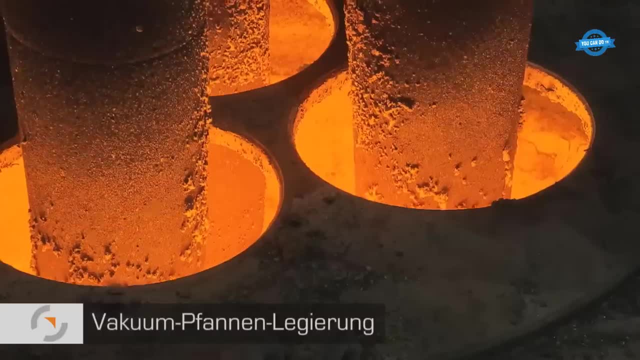 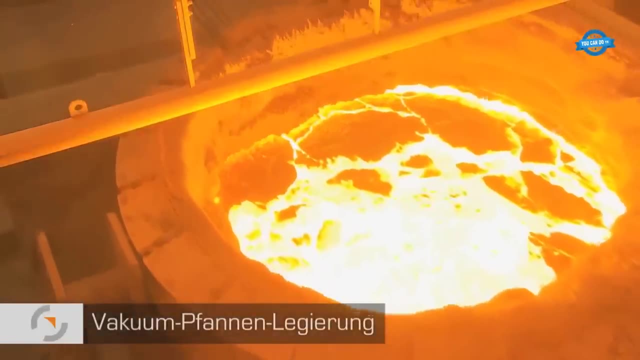 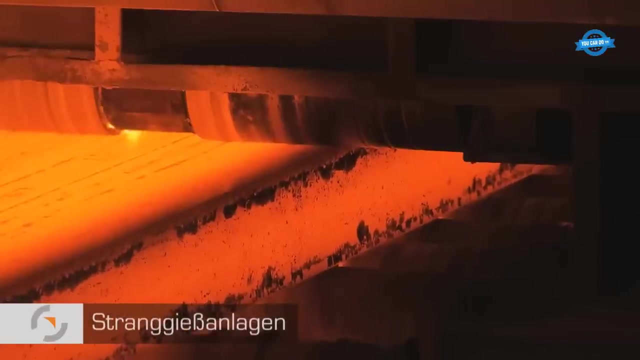 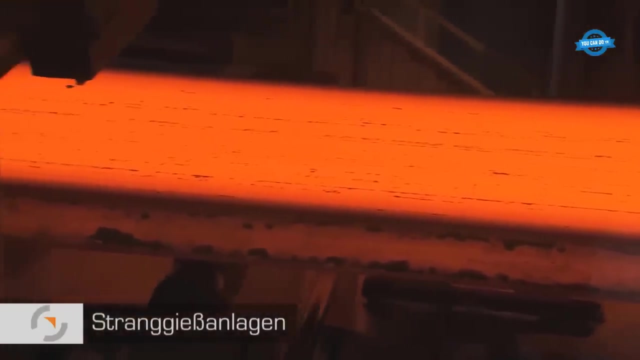 vacuum chamber to remove any remaining impurities. This process results in a cleaner and higher quality steel. After the VLA treatment, the steel is sent to the continuous casting plants, where it is cast into slabs or billets. This process involves pouring the liquid steel into a water-cooled mold, which then solidifies. 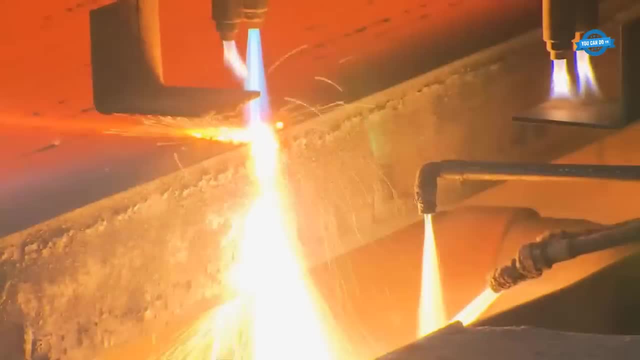 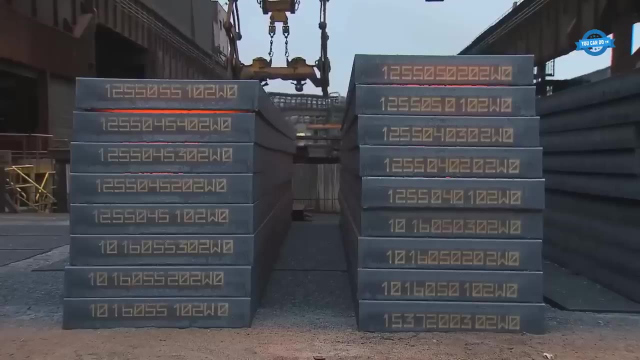 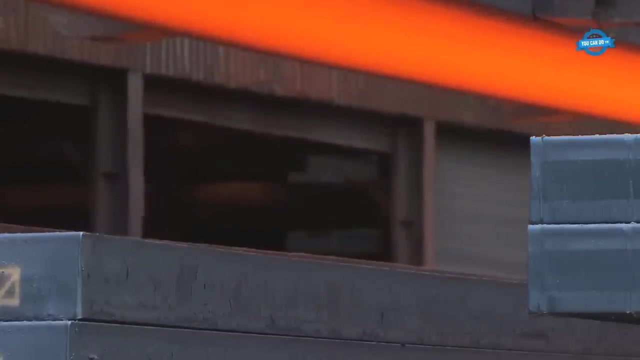 the steel into a semi-finished product. Continuous casting is a highly efficient process, as it eliminates the need for intermediate steps such as ingot casting, which were used in traditional steel production. It also produces a higher quality steel product with consistent properties, resulting in less 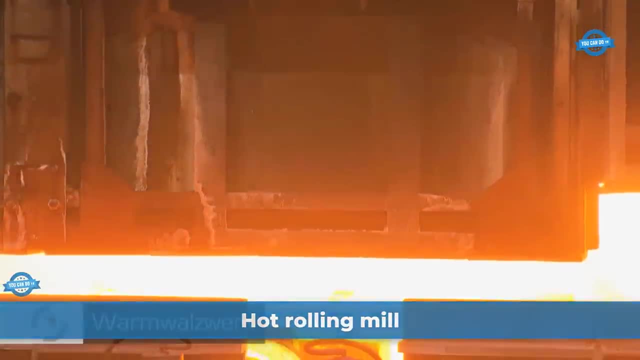 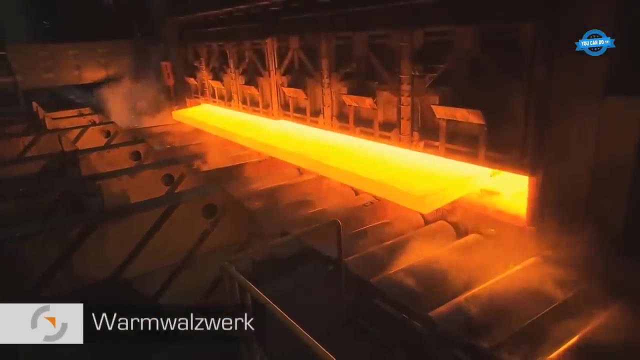 waste and increased productivity. The hot rolling mill is designed to produce steel slabs up to 250 millimeters thick and 2.1 meters wide. It uses a reheating furnace to heat the steel slabs to a temperature of around 1,200 degrees. 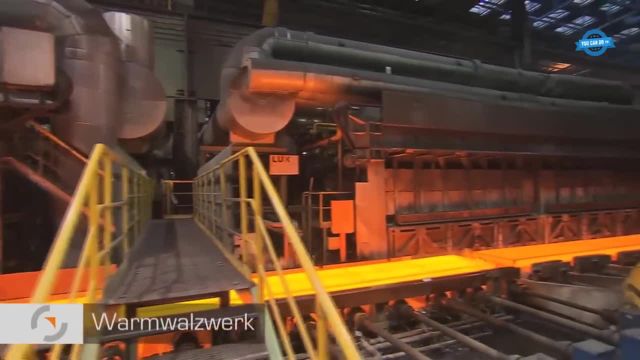 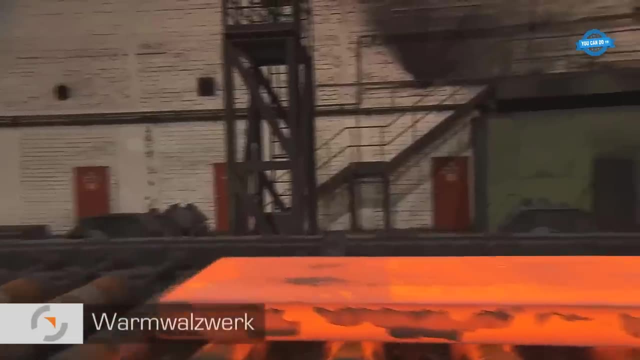 Celsius, which makes them soft and malleable. The slabs are then passed through a series of rolling stands, which gradually reduce their thickness and shape them into coils. The hot rolling mill can produce up to 3.5 million tons of steel per year. 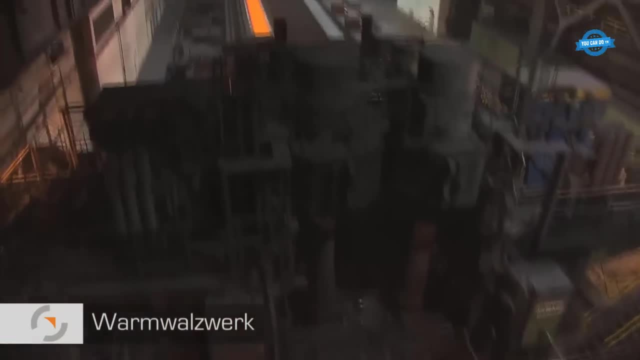 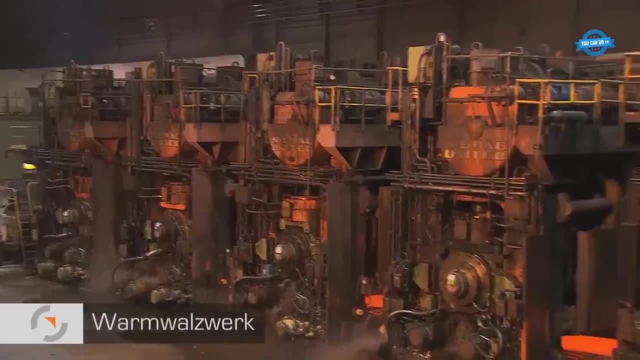 The hot strip line processes the coils produced by the hot rolling mill. The coils are then passed through a series of rolling stands which gradually reduce Those are uncoiled and fed through a series of rollers which reduce their thickness to the desired level. 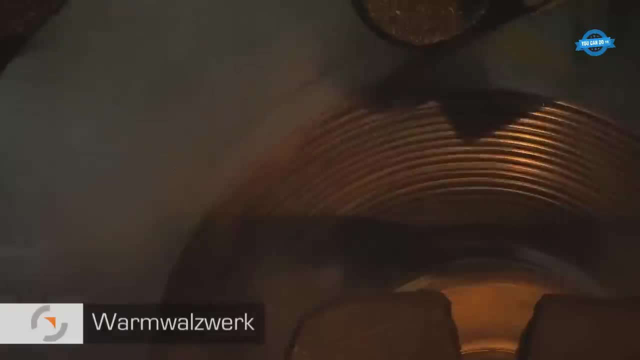 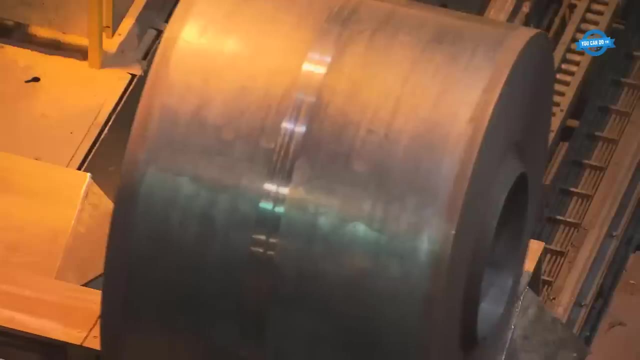 The hot strip line can produce steel strips up to 1,850 mm wide and 20 mm thick and can process up to 4.5 million tons of steel per year. The pickling line at Salzgitter AG is used to remove impurities and oxide layers from. 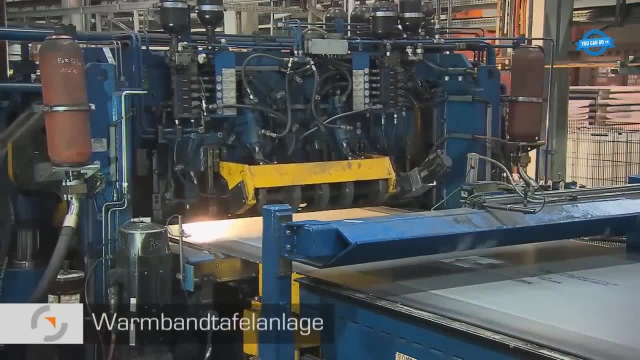 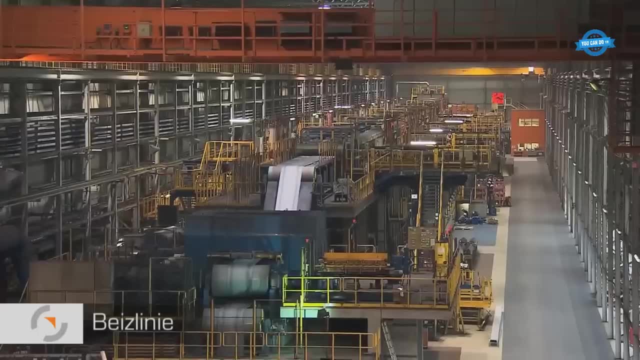 the surface of the steel strips produced by the hot strip line. The strips are passed through a bath of hydrochloric acid, which dissolves the impurities and leaves the surface clean and smooth. The pickling line can process up to 1.8 million tons of steel per year. 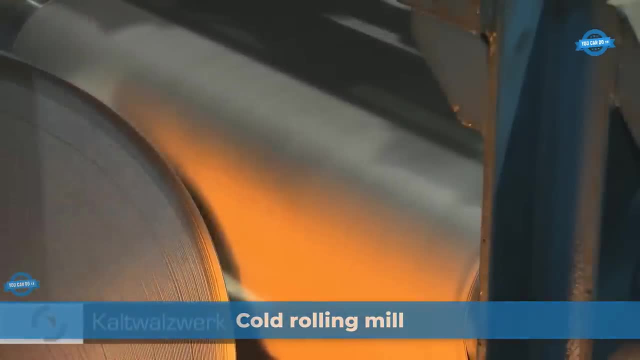 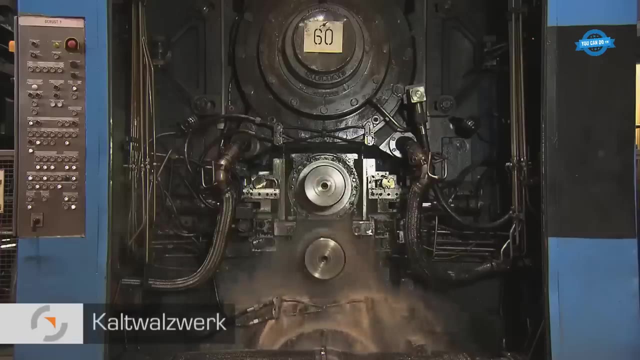 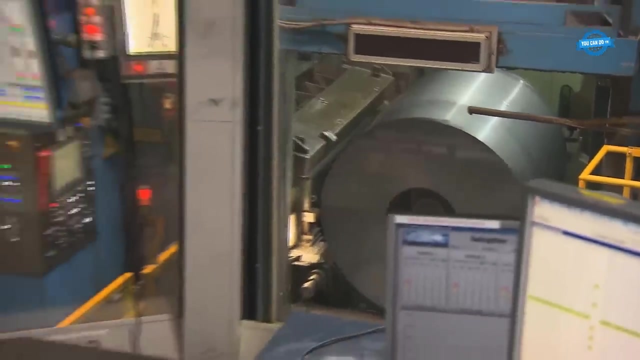 The cold rolling mill at Salzgitter AG is responsible for reducing the thickness of steel coils produced in the hot strip mill to the desired thickness. The process at the cold rolling mill starts with the uncoiling of the steel coils and running them through a series of rollers, gradually reducing the thickness of the steel. 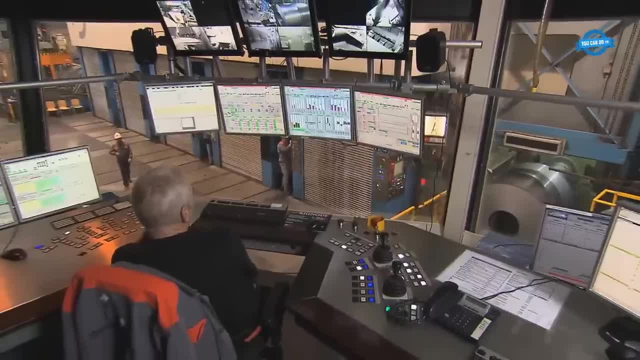 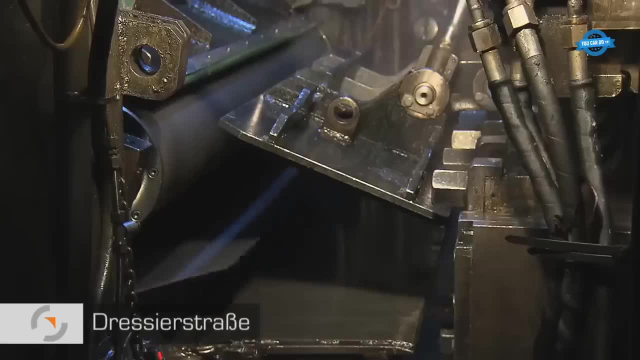 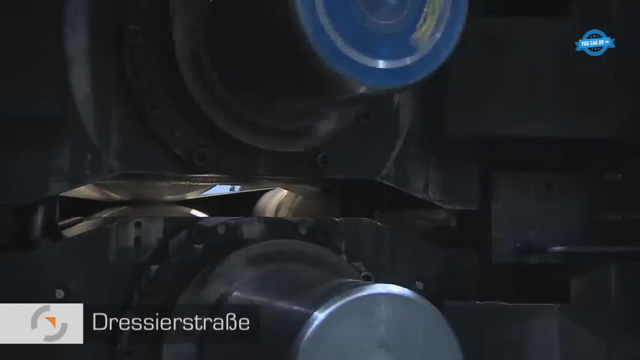 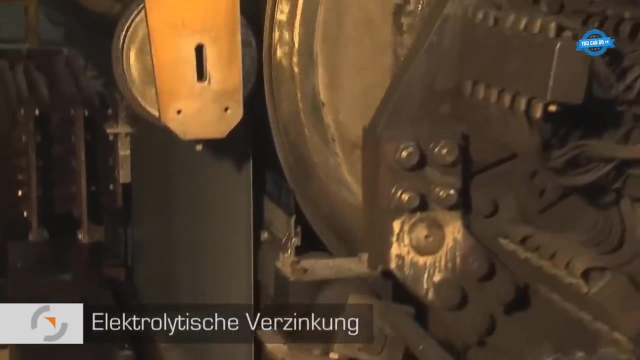 The steel is then recoiled into a new coil at the desired thickness. The cold rolling mill can produce steel coils with thicknesses ranging from 0.3 mm to 3.0 mm and widths of up to 1,600 mm. The cold rolling mill at Salzgitter AG is designed to operate at high speeds, allowing 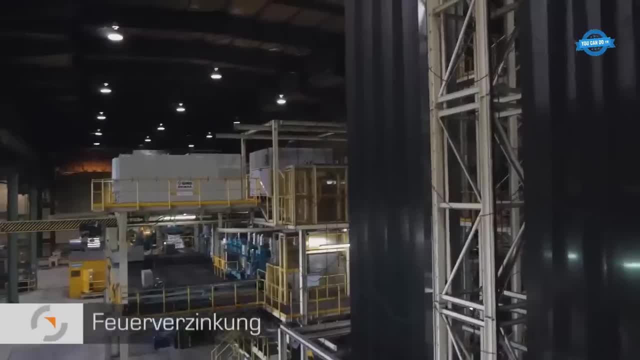 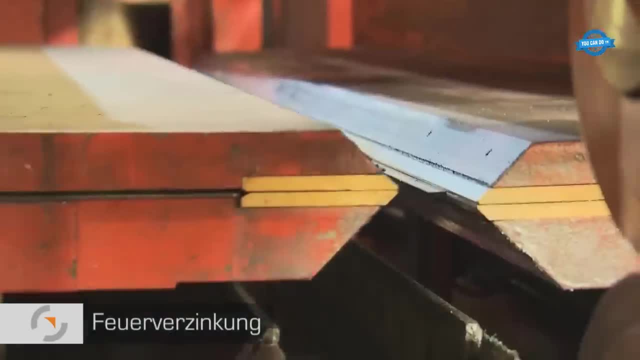 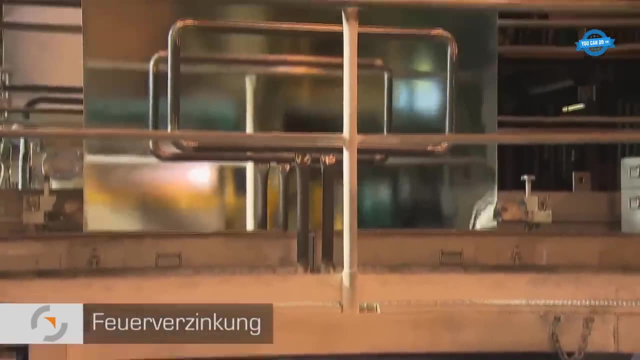 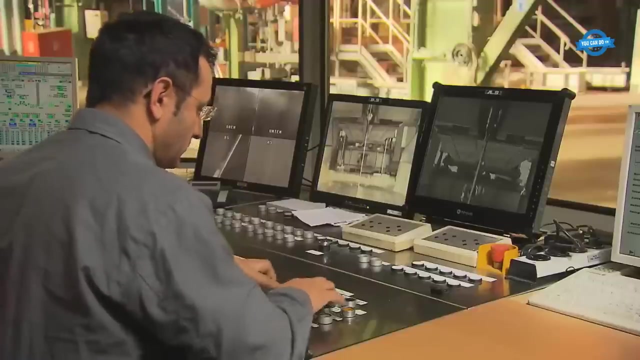 million tons of cold rolled steel per year, making it one of the largest facilities of its kind in Europe. The Cold Rolling Mill is also equipped with a skin pass mill and an electrolytic galvanizing line. The skin pass mill is used to impart a uniform surface finish to the steel coils, while 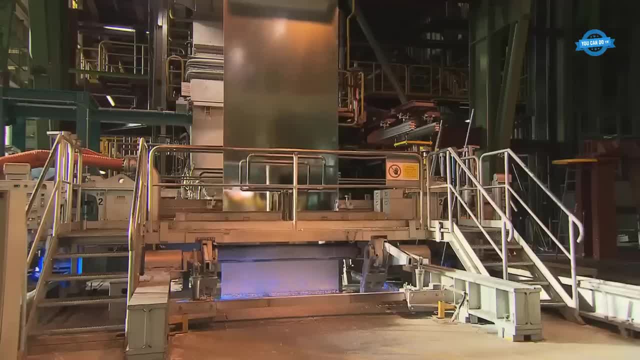 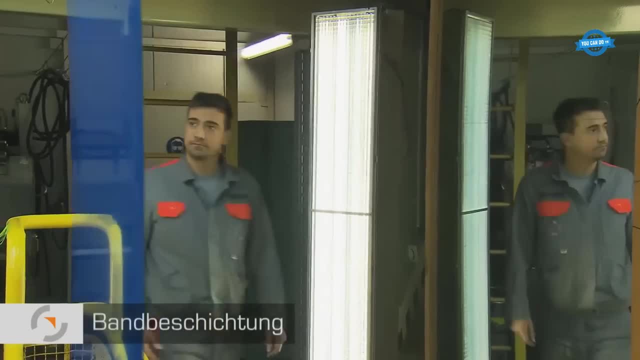 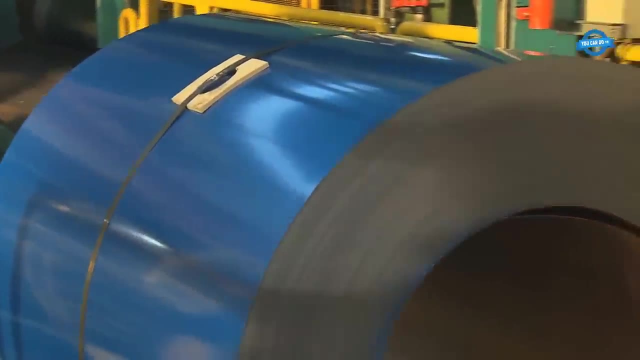 the electrolytic galvanizing line applies a layer of zinc to the surface of the steel to provide corrosion protection. These additional processes enhance the quality and durability of the product and make it possible for this mill to be processed. the steel products produced at Salzgitter AG. 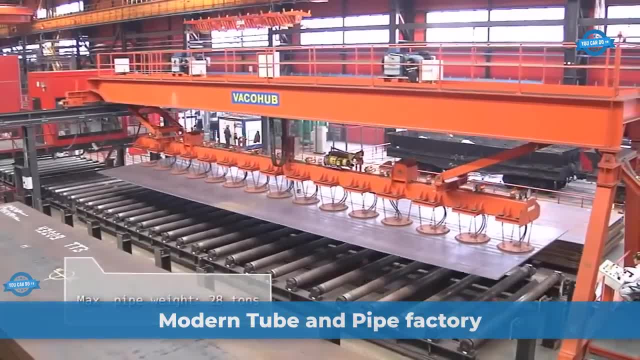 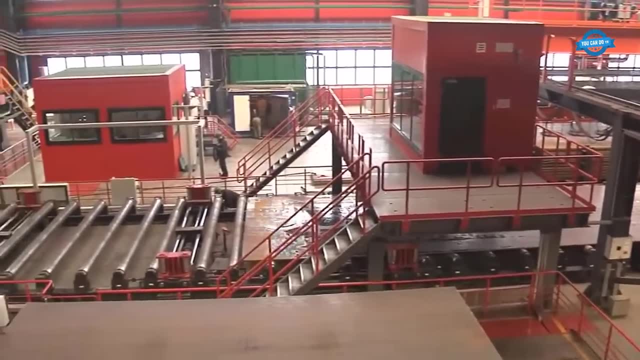 OAO Chelyabinsk, or Chelpipe, is a Russian company that produces welded and seamless steel tubes and pipes for the oil and gas industry. The production process at Chelpipe begins with the plate infeed unit, where plates are fed into the system. The plates are then. 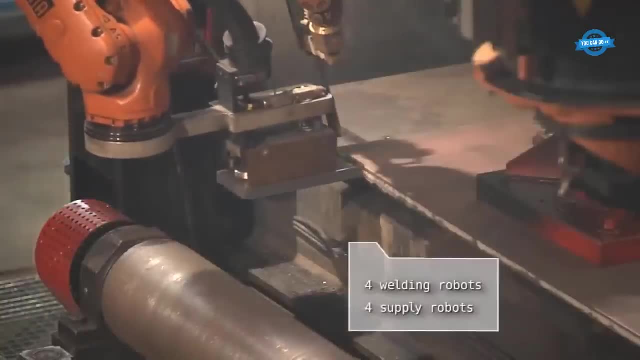 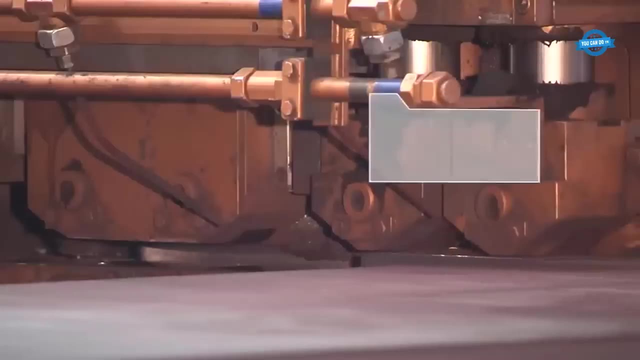 tested using ultrasonic testing and sandblasting units to ensure their quality. After testing, the plates move to the automatic tab welding station, where they are welded together. The plate edge milling machine and plate edge crimping press are then used to create parallel. 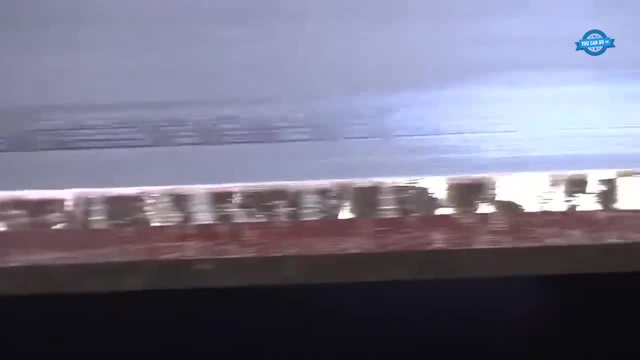 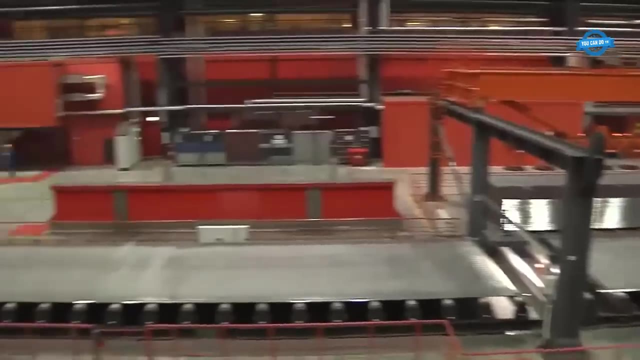 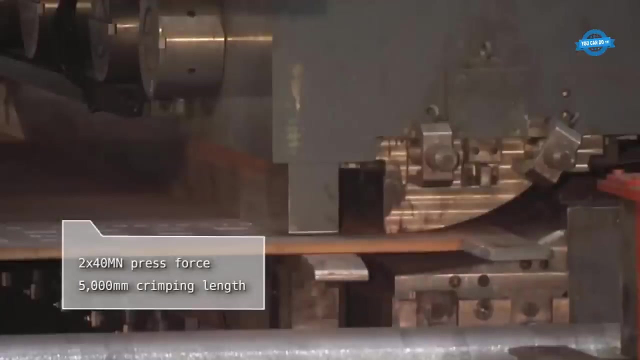 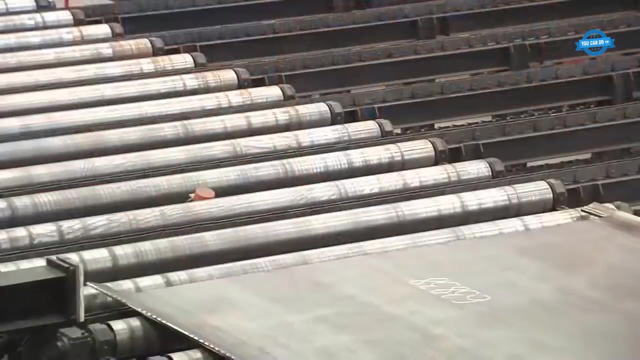 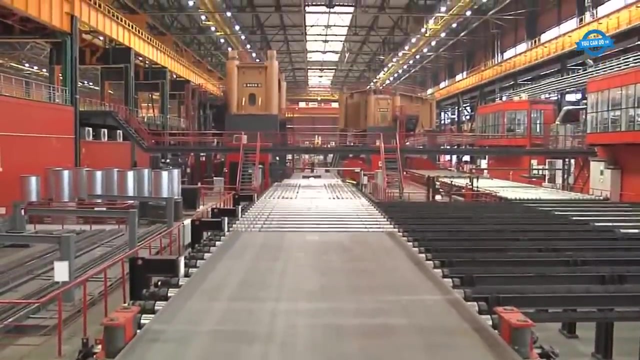 plate edges and beveling tolerances that result in perfect weld seams during final welding. The heart of the plant is the 12-liter GCO pipe forming press and the 18-meter JCO pipe forming press, which allow Chelpipe to adapt its production flexibly in line with demand. 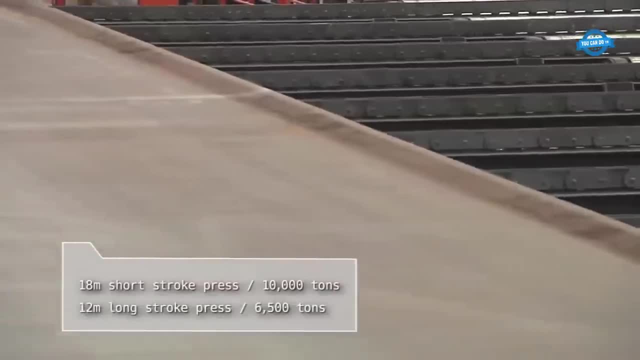 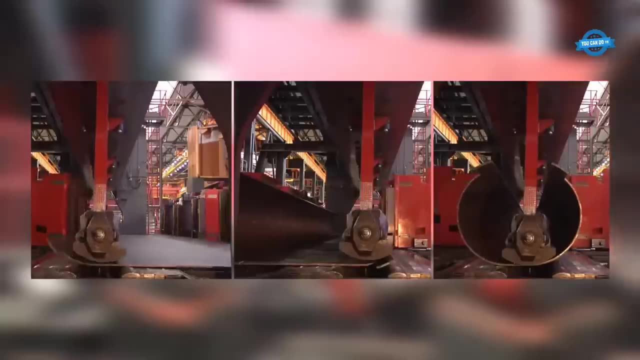 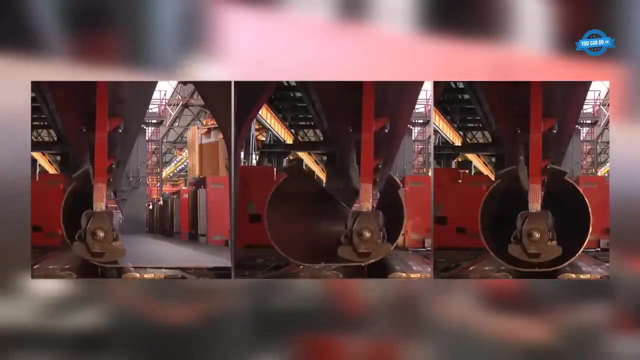 The step-by-step forming process requires only low forces and allows reliable forming even with irregular plate properties. The large press is ideal for the production of 18-meter pipes, which are typically used in Russia for long overland pipelines. More sophisticated offshore dimensions with small diameters and high wall thicknesses are best produced on. 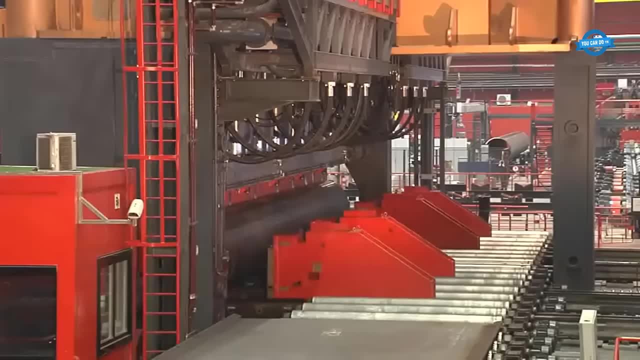 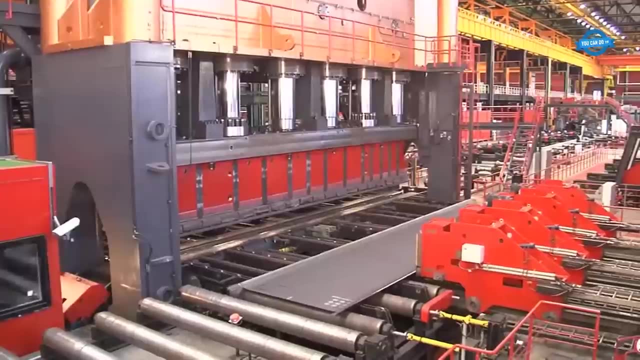 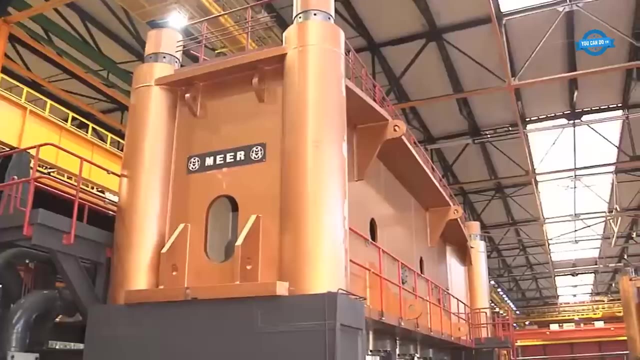 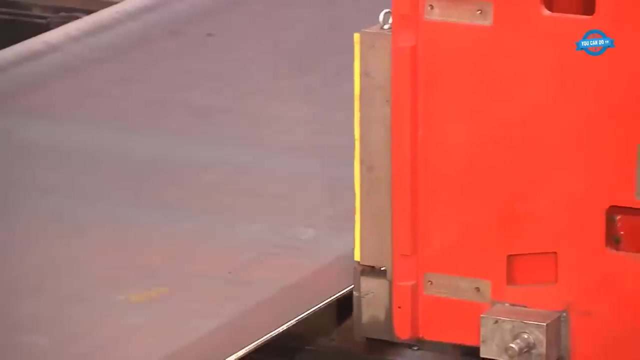 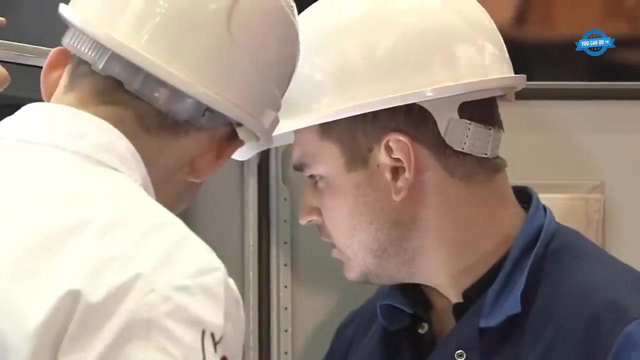 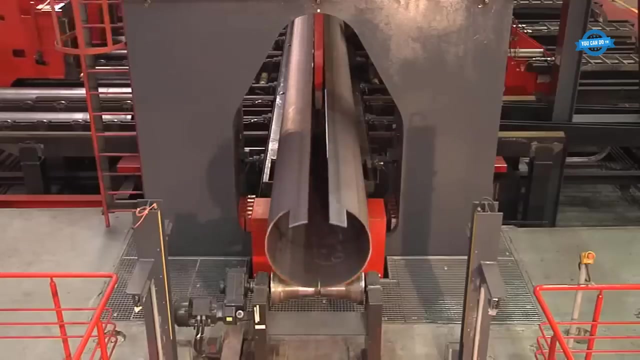 the 12-meter long stroke press. We have a total of 24,000 hopper collars. Now to test out the maize milling machine. We will use a little bit of our machine'sstuff as a guide. We then repeat the operation until. 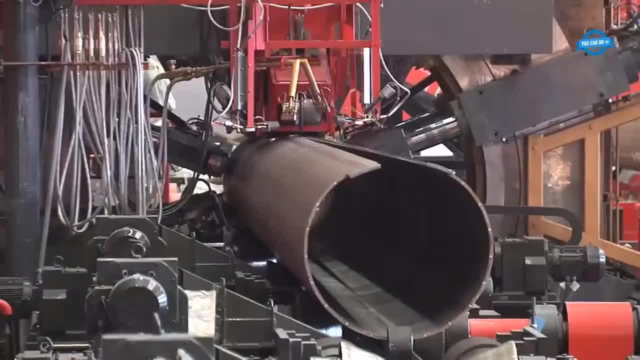 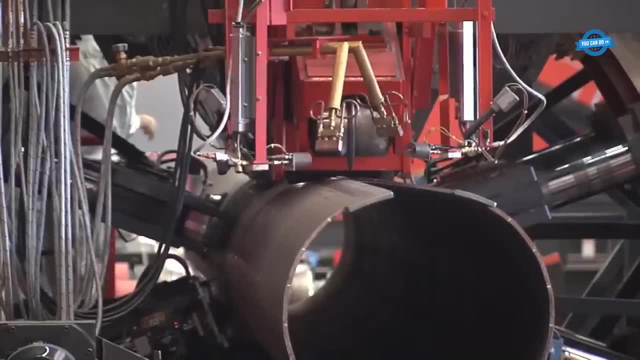 the milling machine is in action, Then we will drop the milling machine onto the running machine immediately after which the milling machine is put on. the" seam pipe is fixed in the downstream tack welding stands, where the hydraulically adjusted roller beams bring the plate edges precisely together In conjunction with the constant feed control. 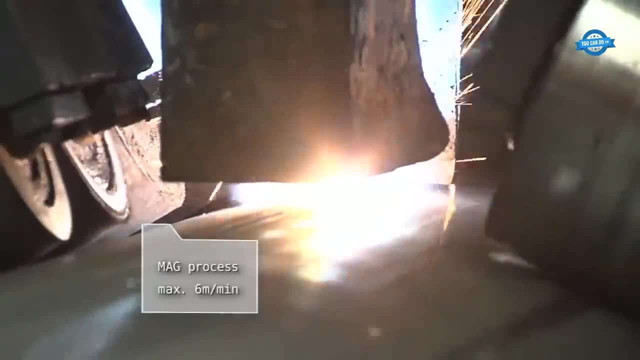 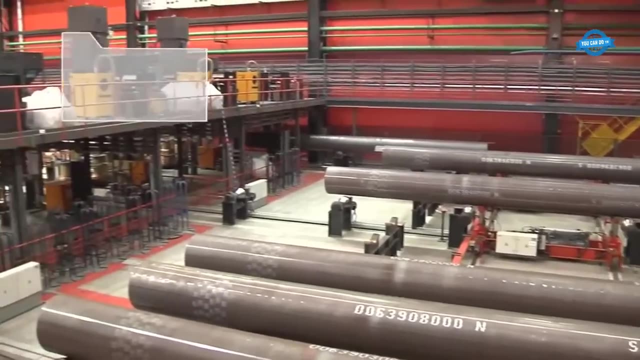 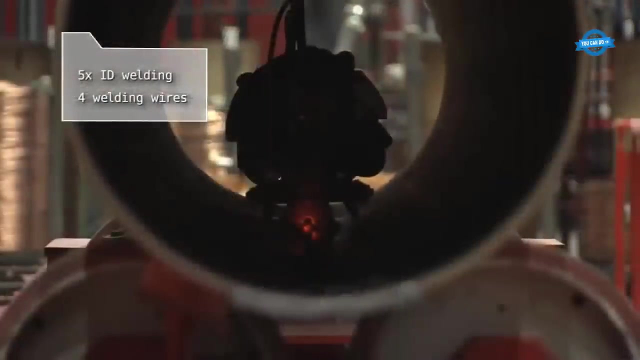 system. this results in a continuous and reliable tack weld. Inside welding uses the submerged arc welding SAW process, which produces uniform weld seams in a smooth and vibration-free process. The SAW process is also used for outside welding, using up to five welding wires to create high 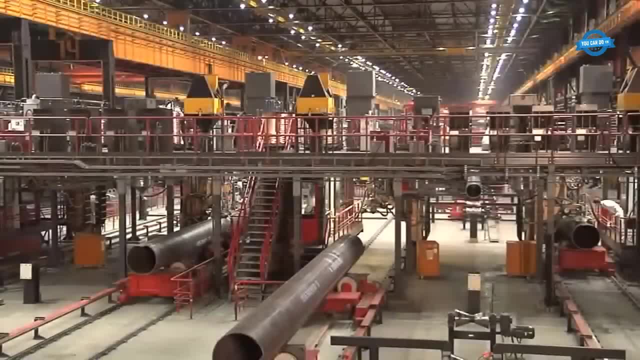 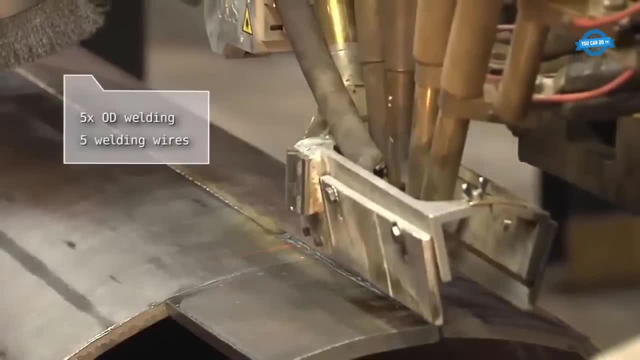 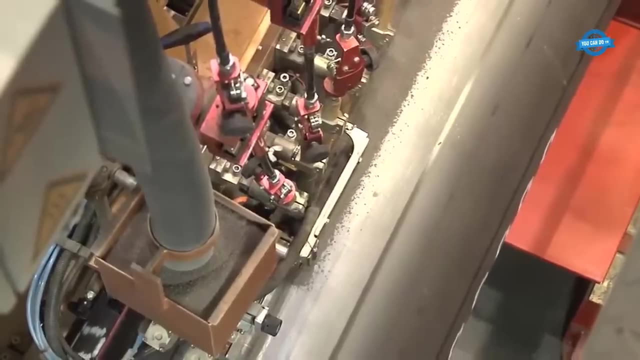 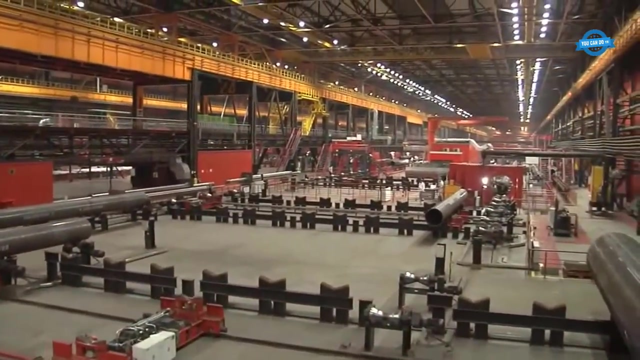 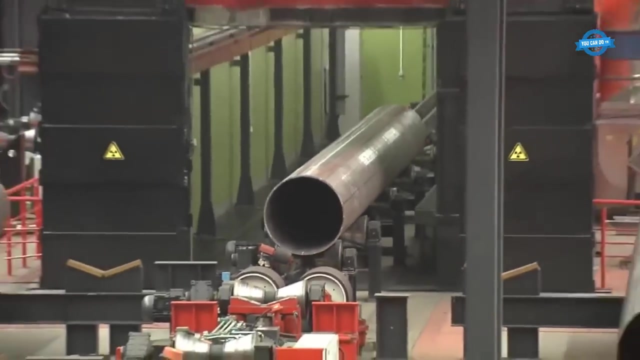 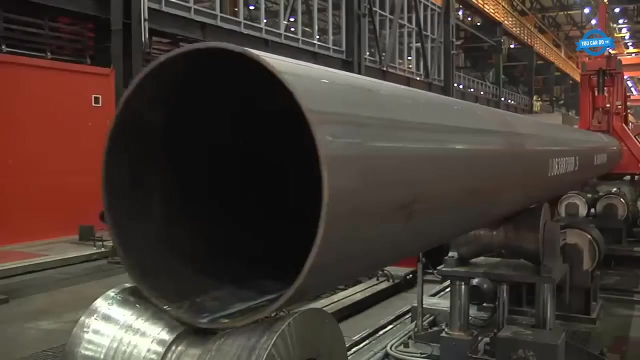 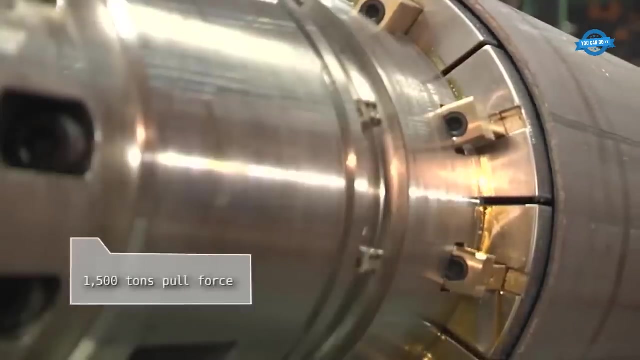 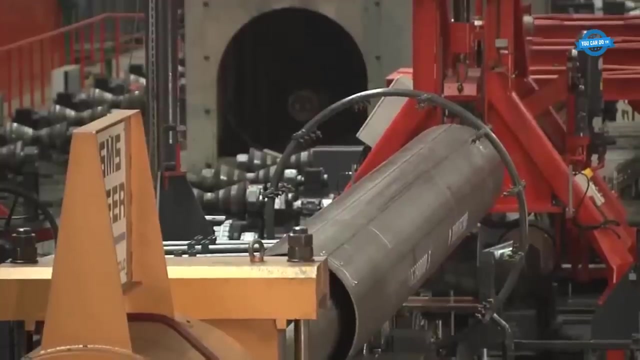 quality welds with flawless seams and good material properties. To safeguard process reliability, the pipe is checked by means of non-destructive testing, using ultrasonic and x-ray testing. Pipe calibration with two mechanical expanders is then used to simultaneously size and straighten the pipes while improving material properties. 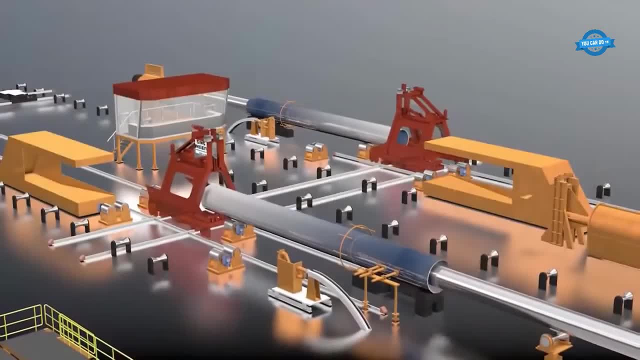 The SMS Mayer expander is known for its high positioning accuracy, and when the two machines are used in parallel, the pipe is checked by means of non-destructive testing. using ultrasonic and x-ray testing In parallel for 12-meter pipes, the highest productivity is achieved. 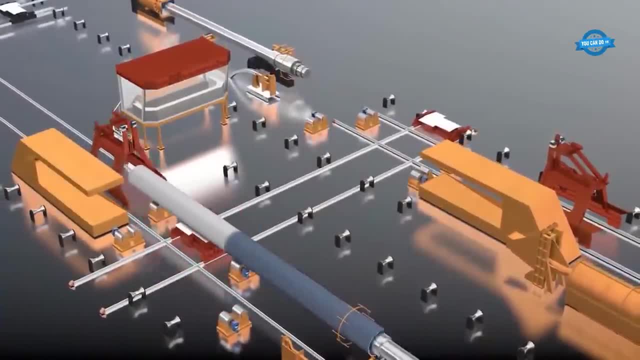 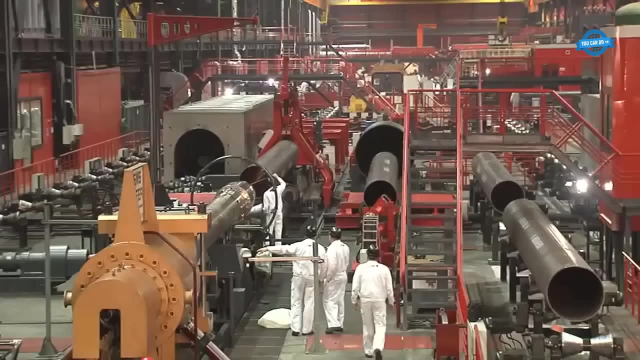 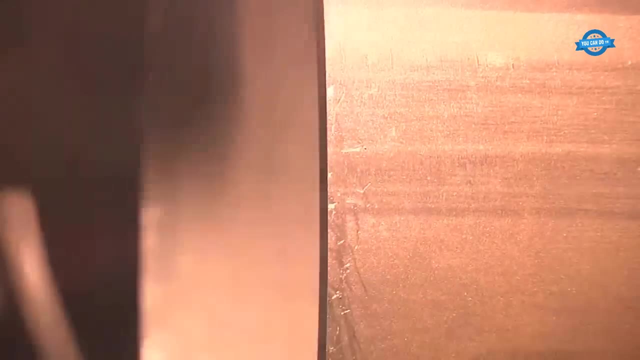 The entire works is controlled by a level 3 automation system supplied by SMS Mayer. This manufacturing execution system is responsible for both pipe tracking and the entire quality assurance and documentation of certified tube and pipe qualities. The plant is not only one of the most modern in the world, but also one of the best in terms of flexibility and performance. 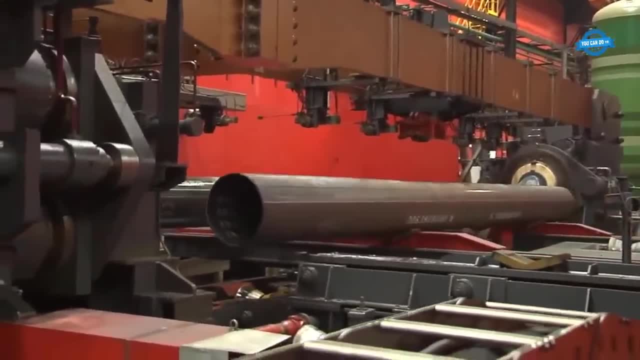 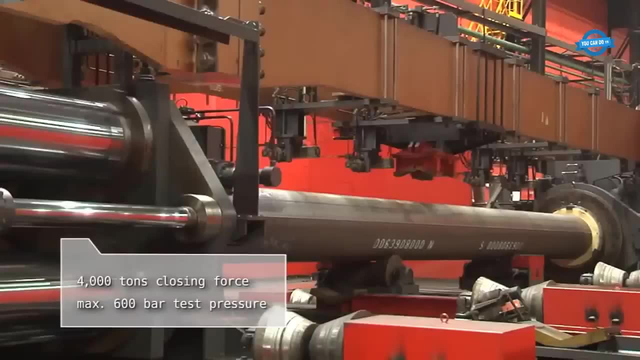 The annual capacity is up to 900,000 tons of pipes, and the plant is designed for a wide range of dimensions and steel grade. Both WhatsApp SMS Mayer and SMS Mayer make use of the best in terms of performance and quality. Since we work with the same company, we mainly focus on using the best types of equipment. 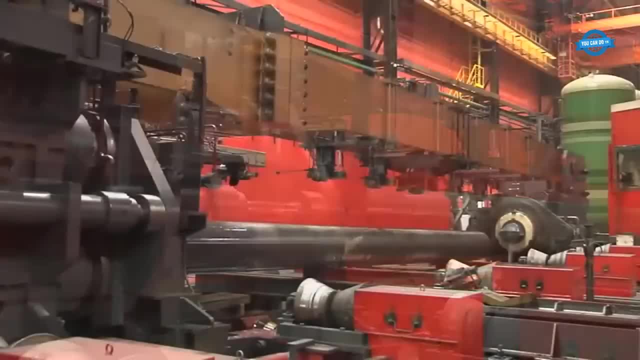 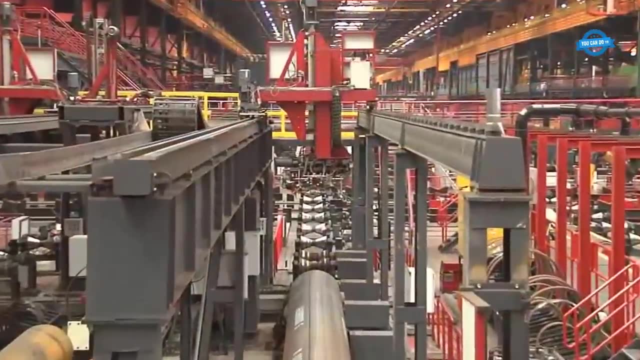 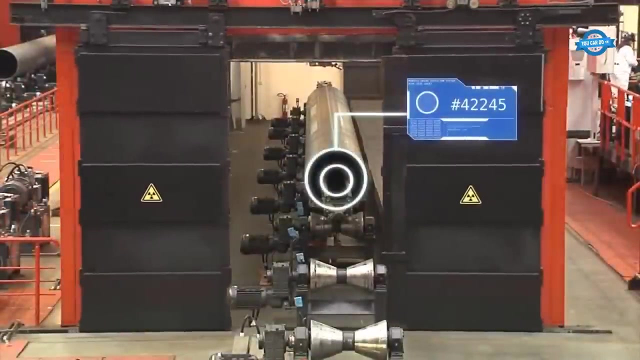 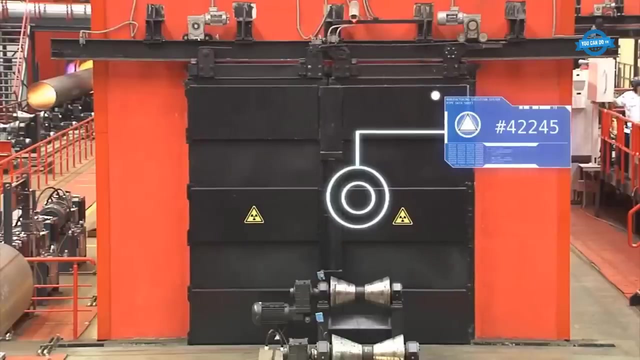 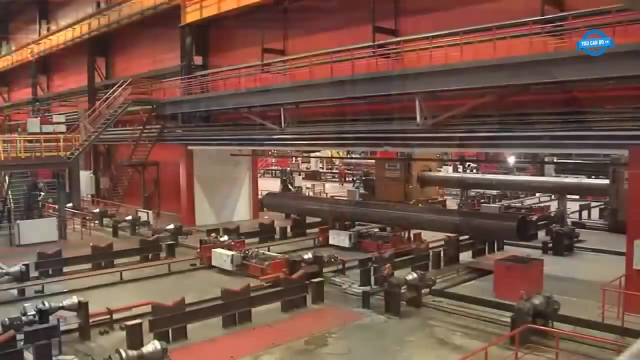 and we are able to improve our specific power warmers By observing the highest quality standards. Chelpipe meets the market requirements and comprehensive service packages ensure long-term plant availability and productivity. SMS Mayer was the general contractor and designed the equipment according to the customer's requirements. 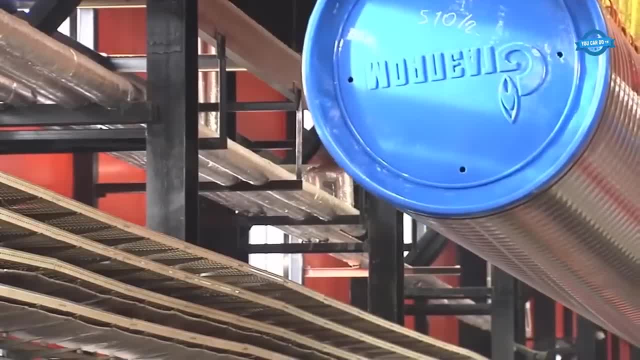 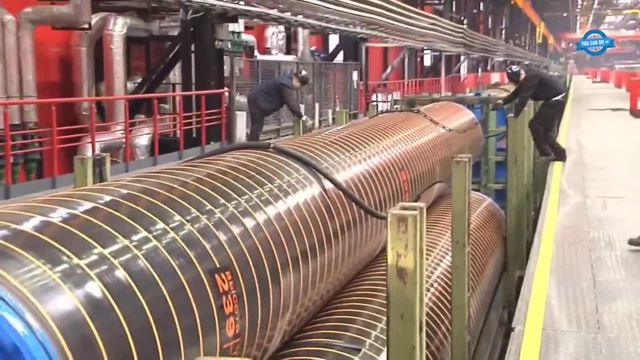 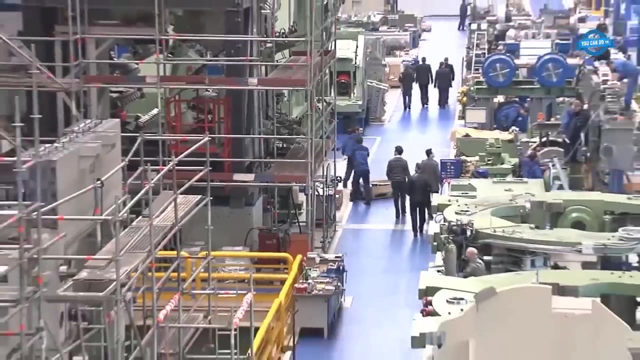 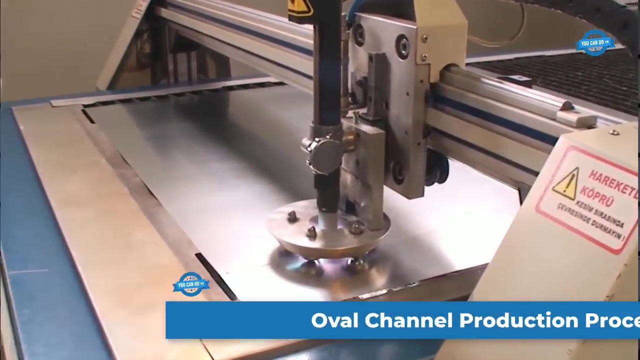 Chelpipe required a supplier who could react flexibly and not just supply standard equipment, but could also meet its requirements and modify the equipment to its specifications. Oval channel production is a specialized process that involves the use of a variety of equipment and techniques to produce high-quality, durable products. 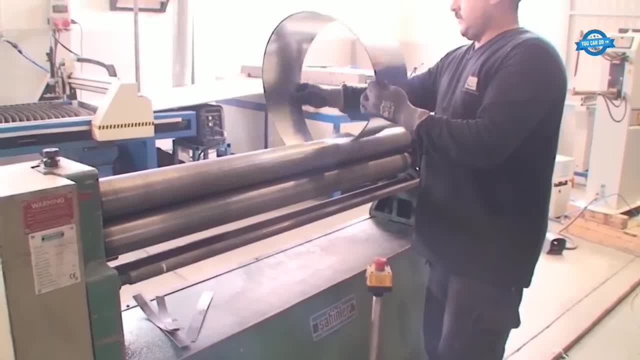 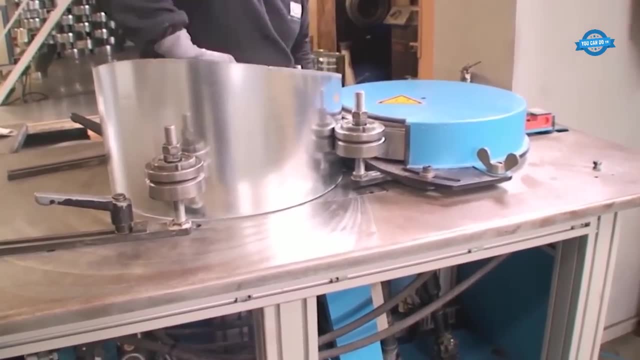 The first step in the oval channel production process is to select the appropriate grade of steel sheet based on the required properties, such as strength and corrosion resistance. Once the steel sheet is selected, it is cut into pieces of the required size using a sheet metal cutting machine. 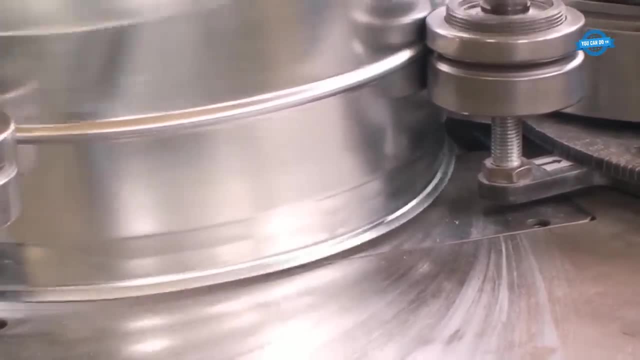 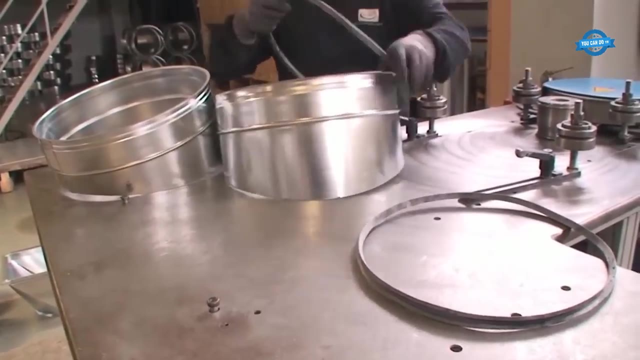 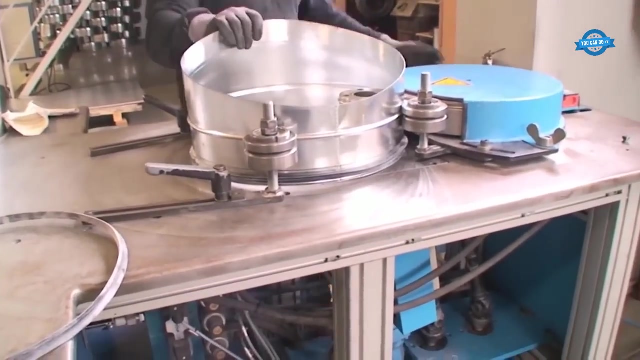 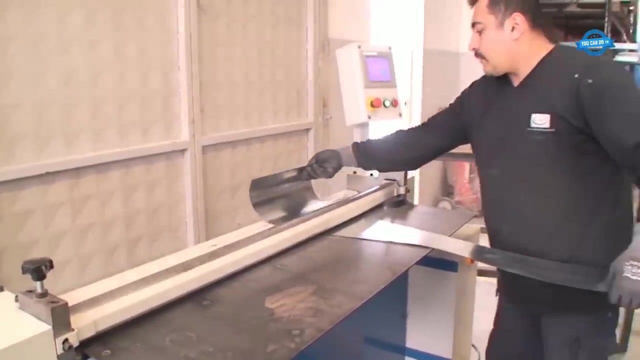 READY TO SELIM. Next, the steel pieces are fed into a bending machine which uses a series of rollers to gradually bend the steel sheet into the desired oval shape. The rollers are adjustable to ensure that the tube is bent to the required dimensions. The bending process ensures 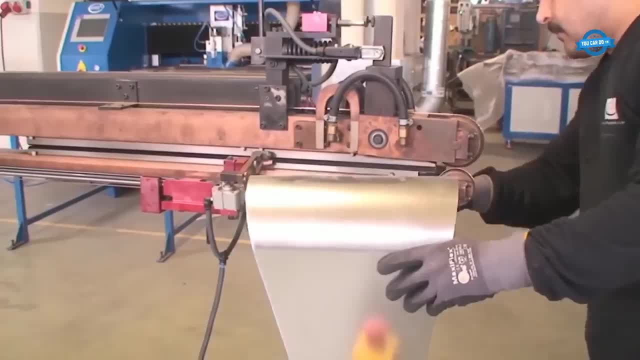 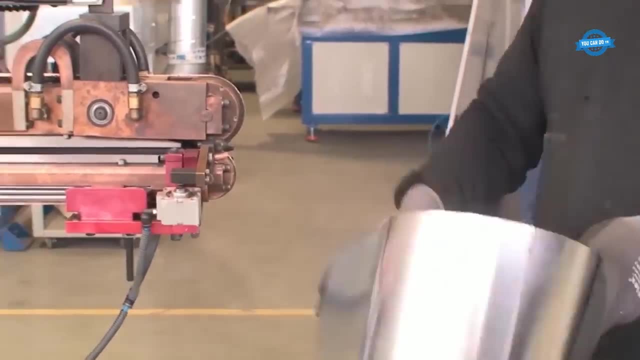 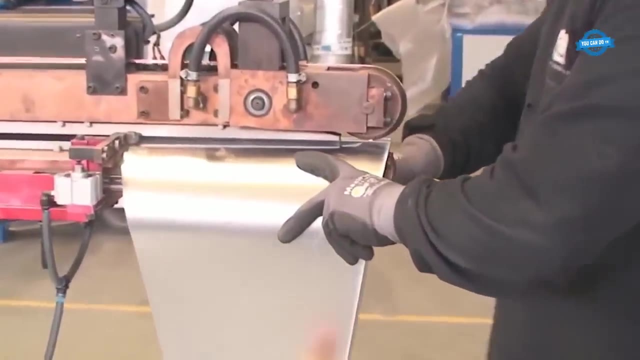 that the oval channels have a consistent diameter and curvature, which is essential for the proper functioning of the final product. After the tube is formed, it is welded using a TIG or MIG welding machine. This welding process ensures that the tube is strong and durable. 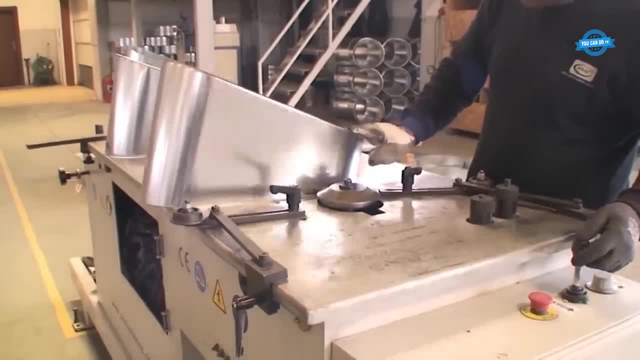 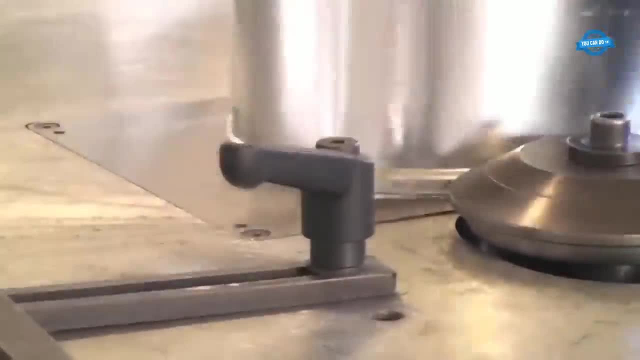 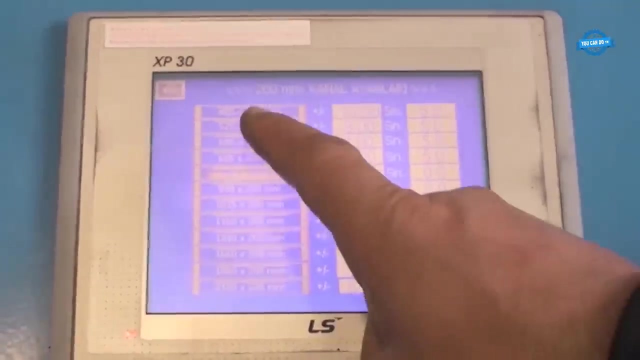 Once the oval channel segments are formed, they are fed into a ribbing and edge forming machine. Sente Machina produces specialized ribbing and edge forming machines that use a combination of rollers and other tools to create the necessary ridges and edges on the oval channels, which improve their structural 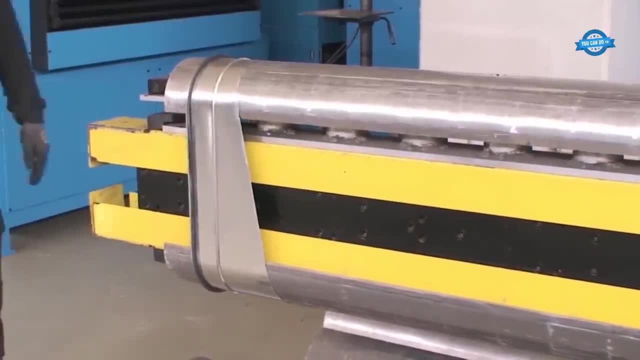 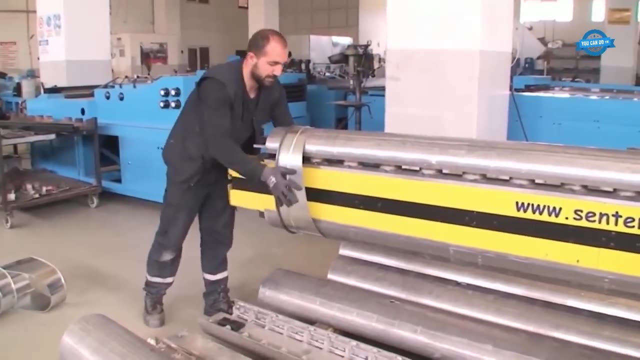 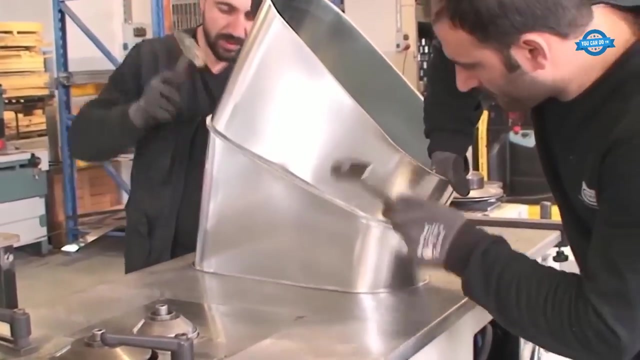 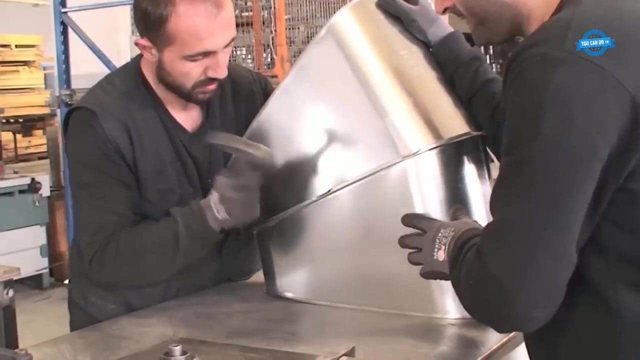 integrity and make them easier to join together. After the oval channel segments have been ribbed and edge formed, they are ready to be assembled together. The connection points between the oval channels are closed using a crimping machine which uses a set of rollers to 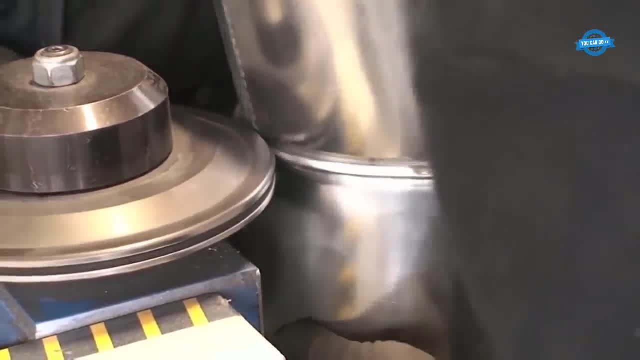 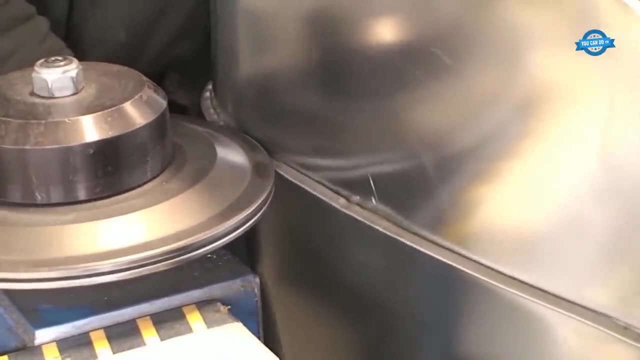 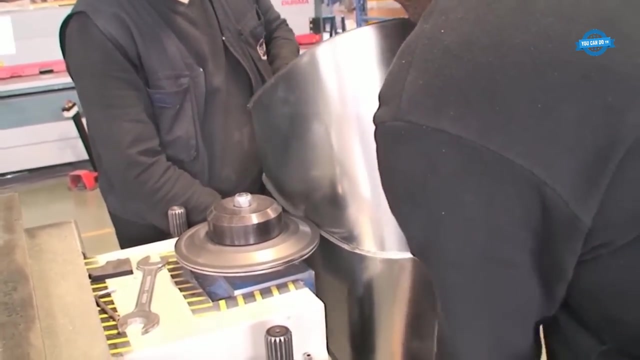 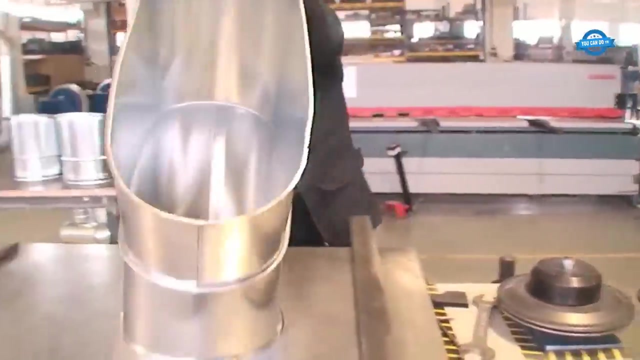 press the connection points together, creating a secure and tight seal. Sente Machina produces a variety of crimping machines that are specifically designed for the oval channel production process, ensuring that the connection points are closed to the required standards. The oval channel production process using Sente Machina offers several advantages over traditional. 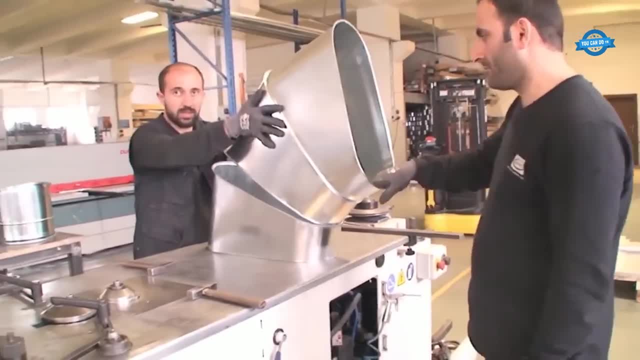 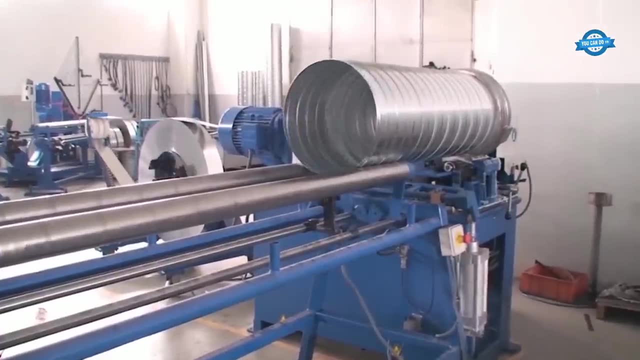 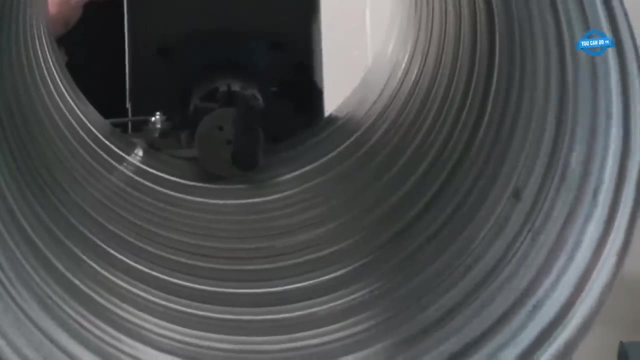 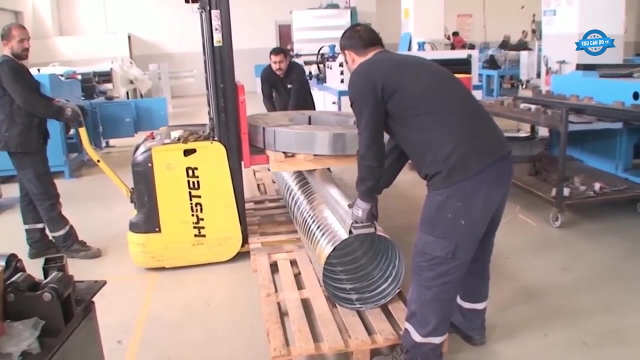 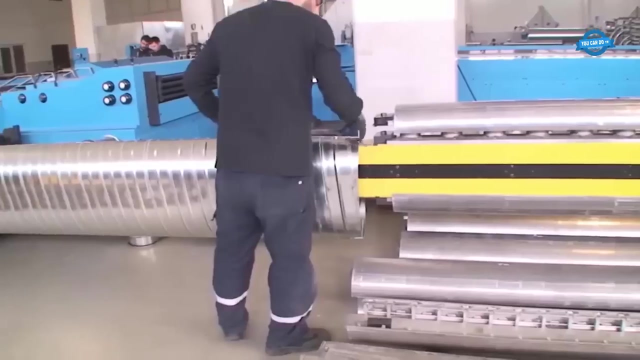 manufacturing methods. One of the most significant benefits is the high level of precision and accuracy that can be achieved. The Sente Machina Machina machine is designed to produce tubes with consistent dimensions, ensuring that each tube is identical to the next. This precision helps to reduce waste and improve efficiency in the manufacturing process. 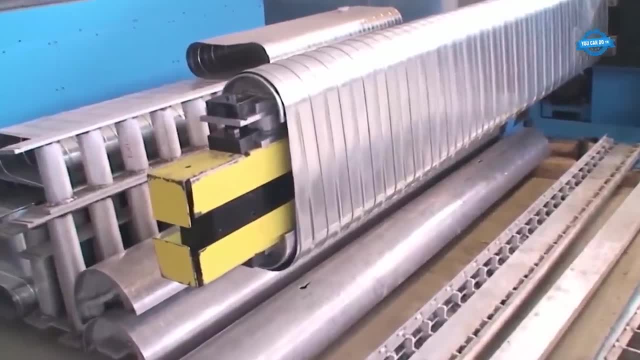 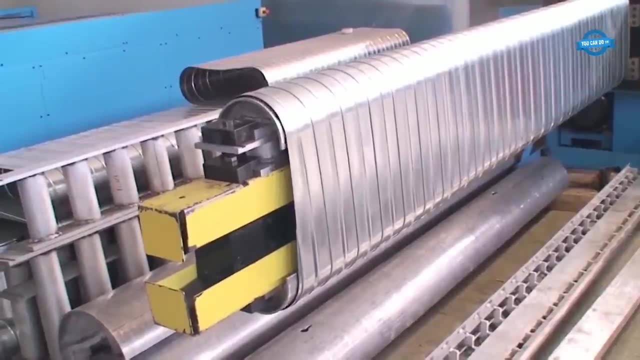 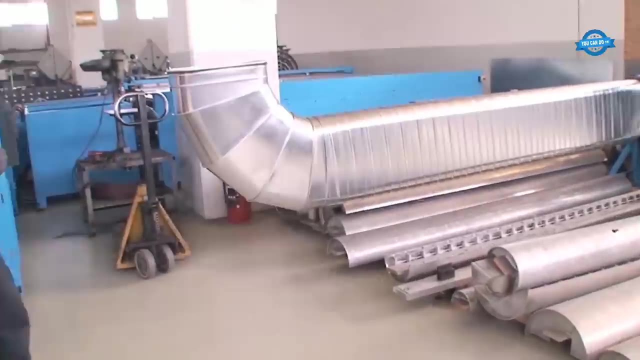 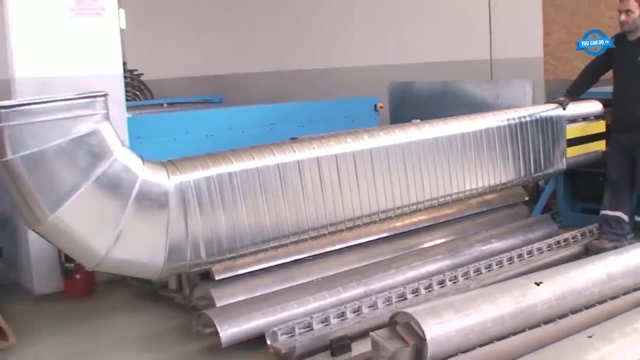 Another advantage of using Sente Machina for oval channel production is the speed of the process. The machines are capable of producing large quantities of tubing in a short amount of time. This makes it possible for manufacturers to meet tight deadlines and production schedules. Makit is a company that specializes in the production of profile drawing machines for 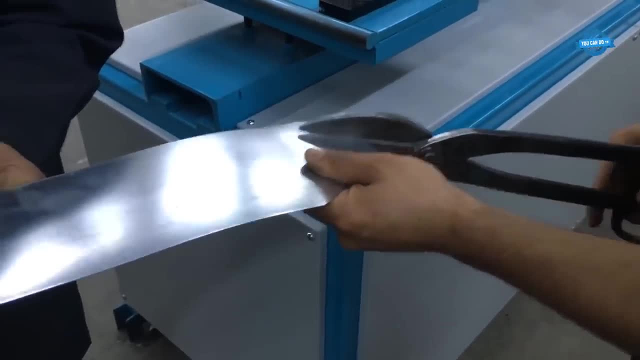 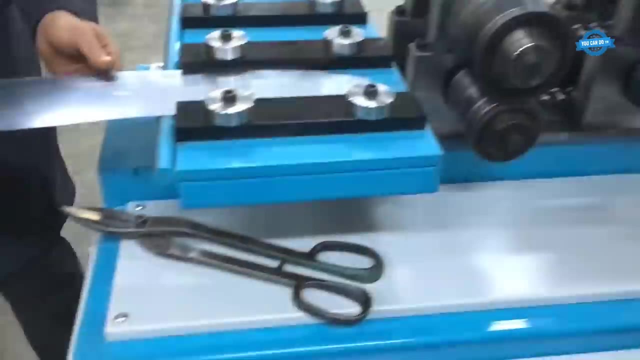 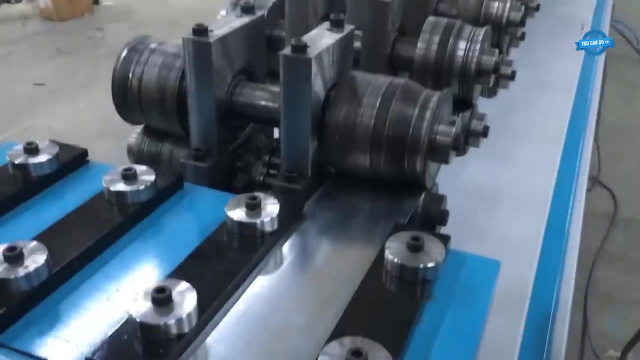 use in the metalworking industry. One of their most popular machines is the Makit 20-30 flange machine. In this section we will explore what a profile drawing machine is and how the Makit 20-30 flange machine works. 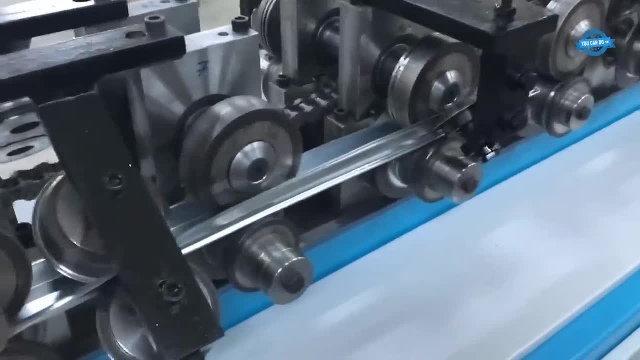 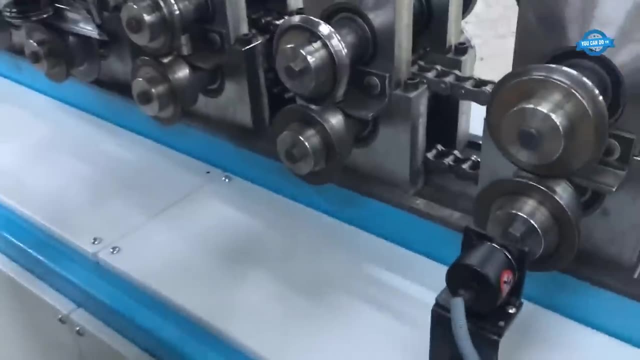 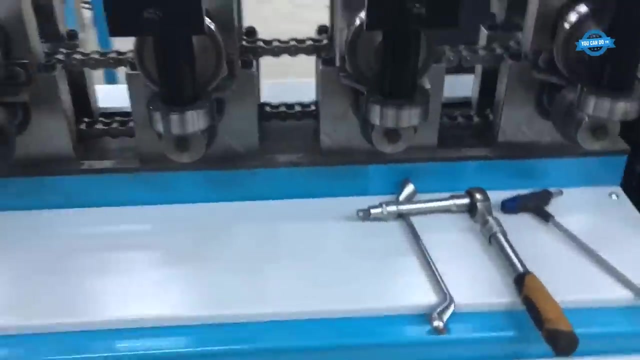 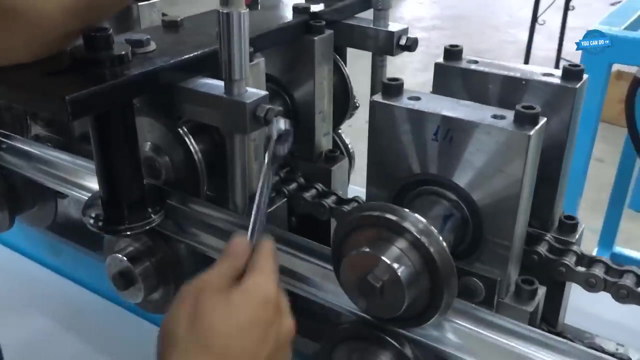 Makit 20-30 flange machine. Profile drawing machines are used to create metal profiles that are used in a variety of industries. The profiles can be made from a variety of materials, including steel, aluminum and copper. The process of creating a profile involves feeding a strip of metal through a set of 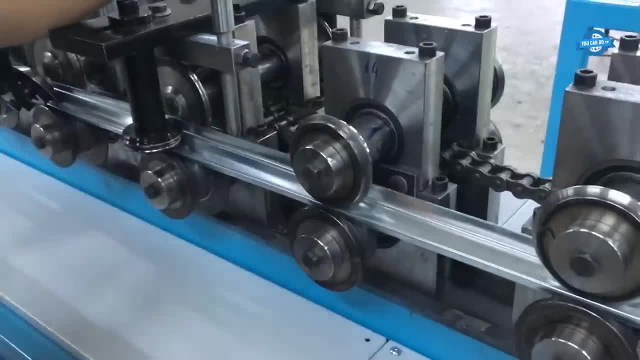 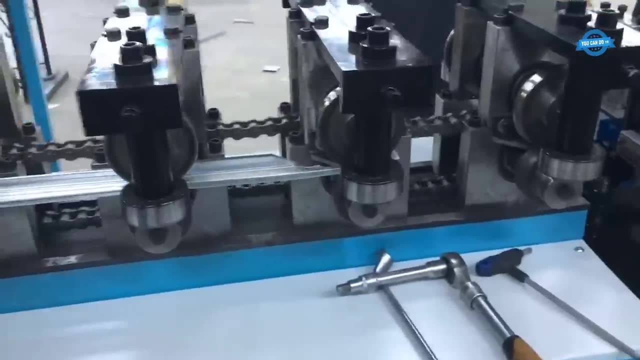 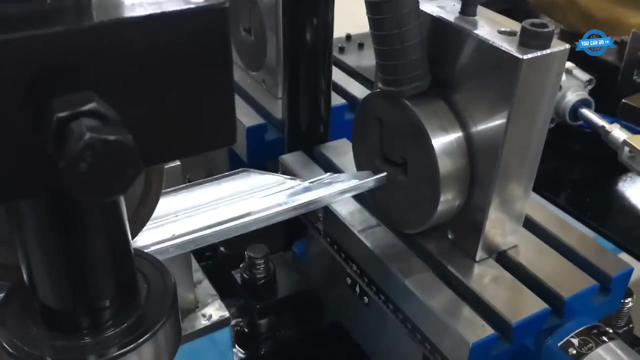 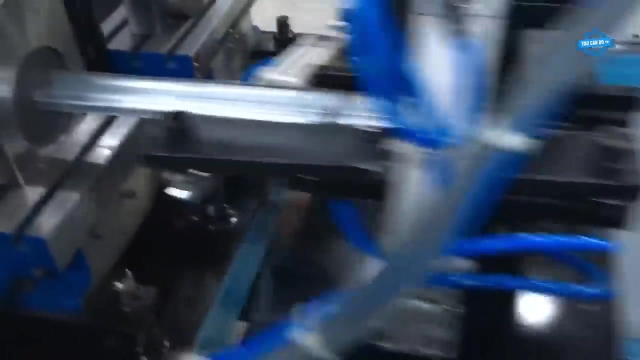 rollers that shape the metal into the desired profile. Makit 20-30 flange machine. Makit 20-30 flange machine. The Makit 20-30 flange machine is a specific type of profile drawing machine that is designed to create flanges. 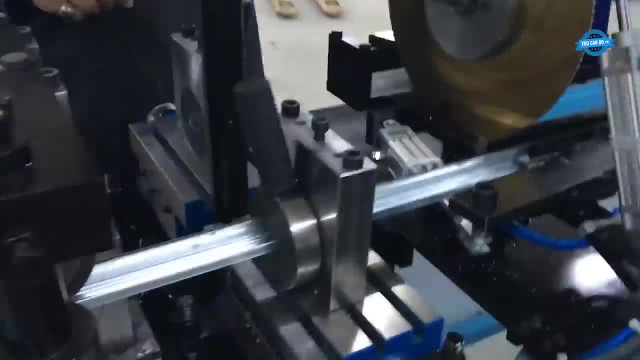 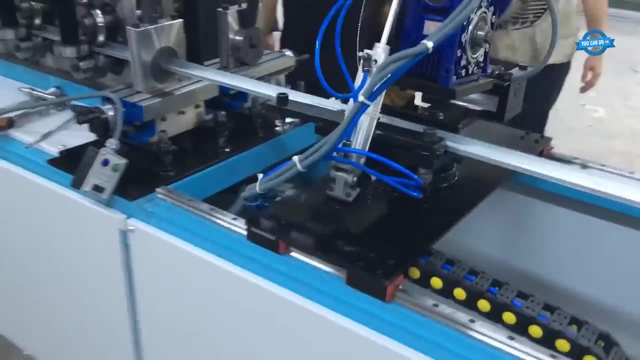 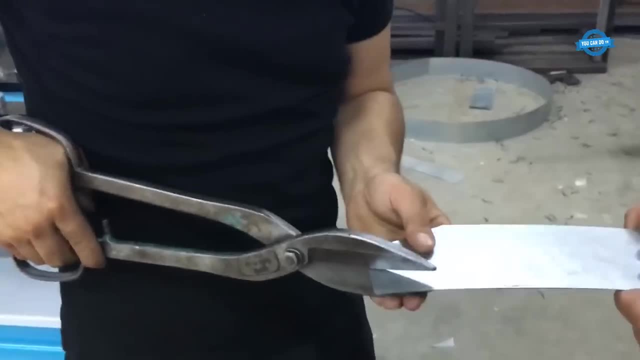 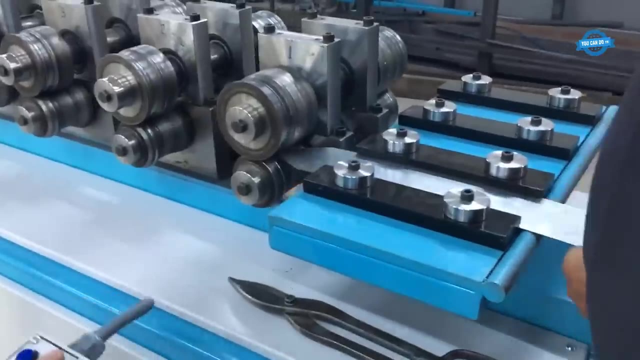 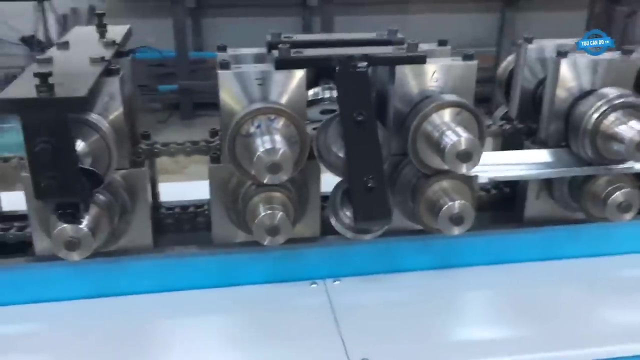 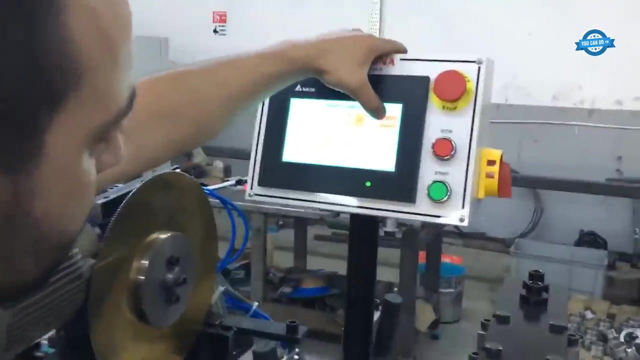 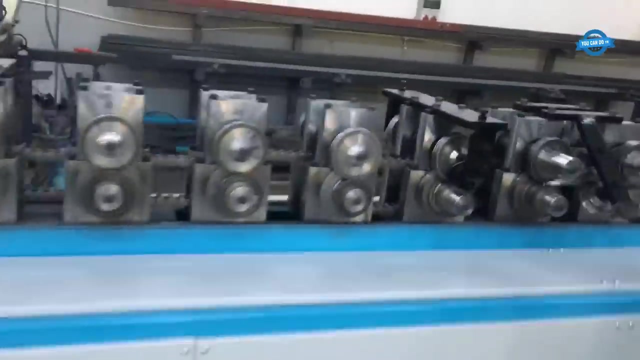 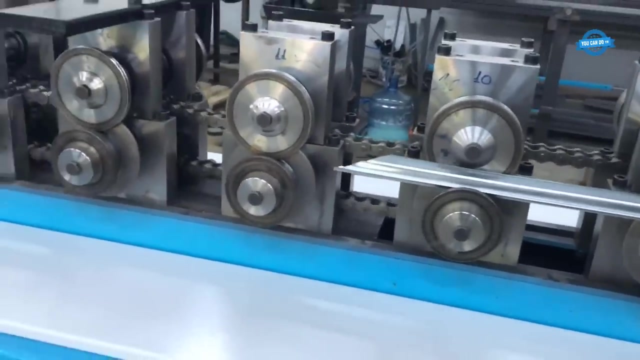 Flange, Flange, Flange. The Maket 20-30 flange machine is a high quality machine that is built to last. It is made from high quality materials and is designed to be durable and reliable. The machine is also easy to use and requires minimal maintenance. 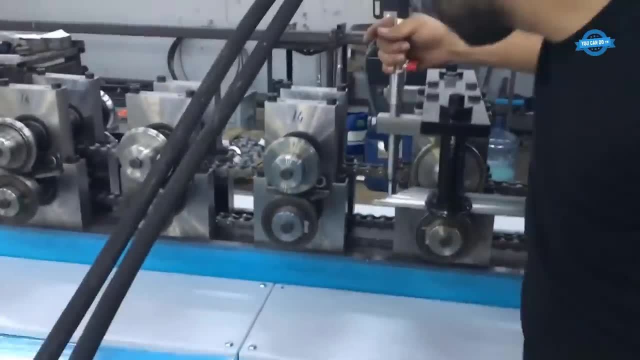 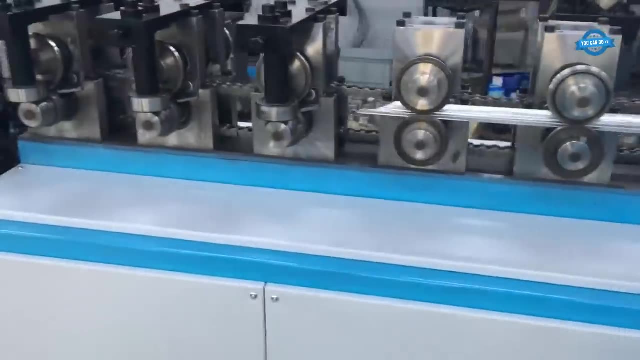 One of the key features of the Maket 20-30 flange machine is its ability to produce high quality flanges quickly and efficiently. The machine is designed to work at high speeds, Which means that it can produce a large number of flanges in a short amount of time. 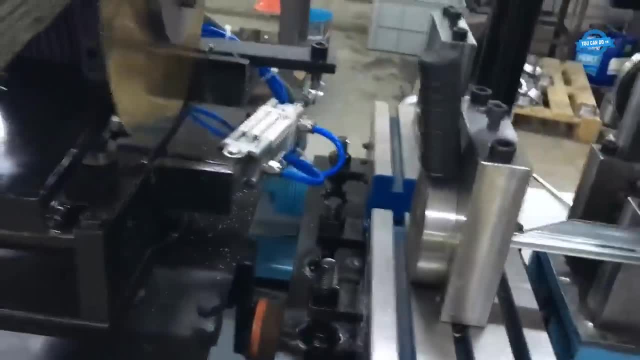 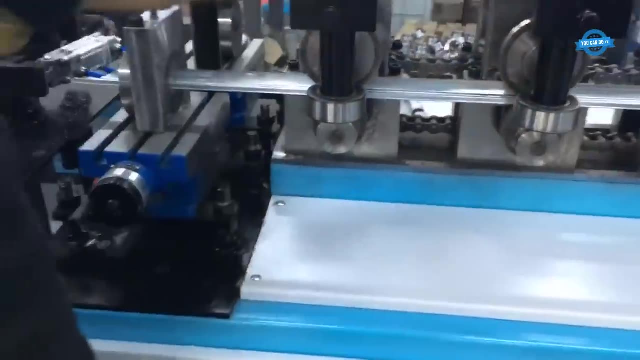 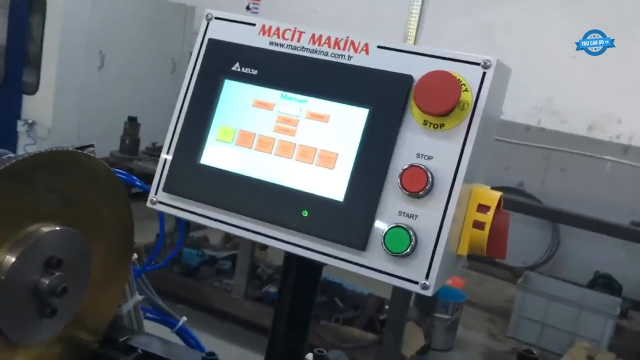 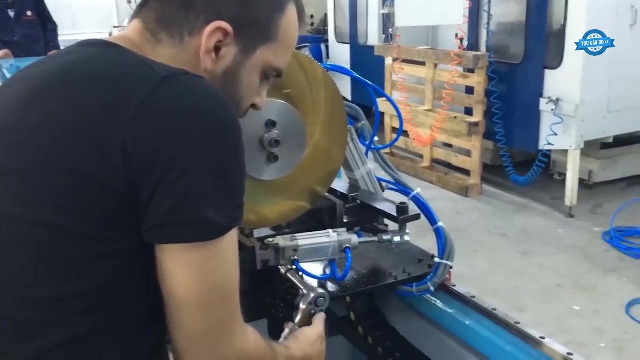 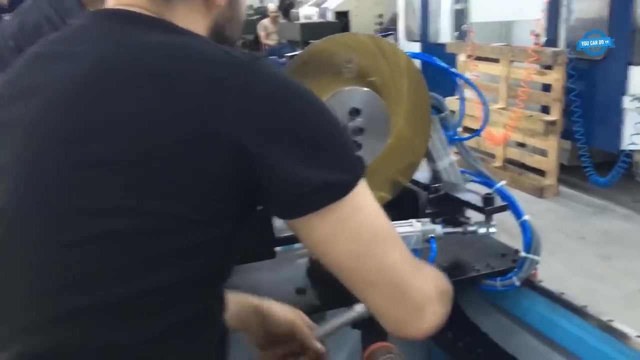 This makes it an ideal choice for companies that need to produce a large number of flanges on a regular basis. The machine is also designed to be easy to set up and use. It comes with a user friendly interface that allows operators to quickly and easily program. 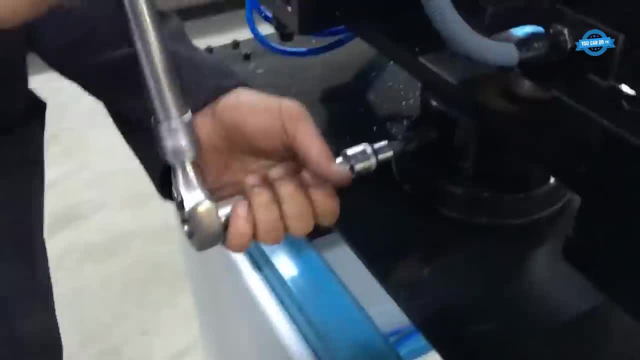 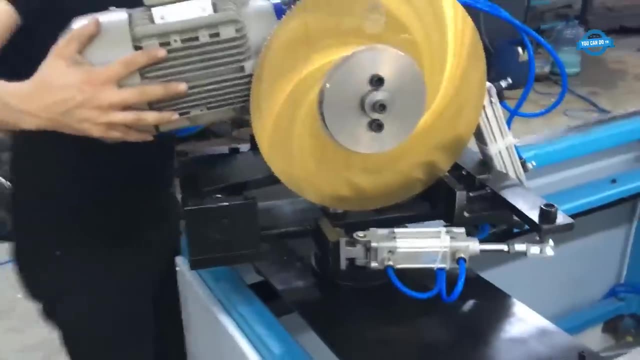 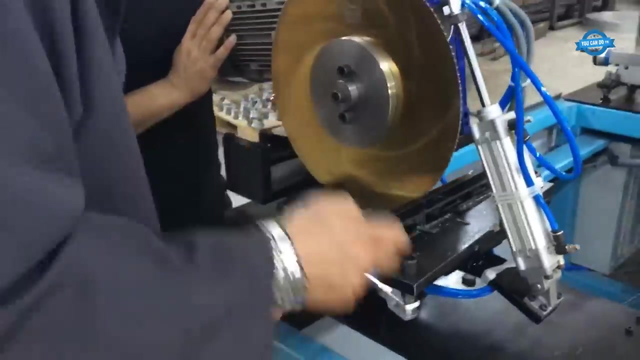 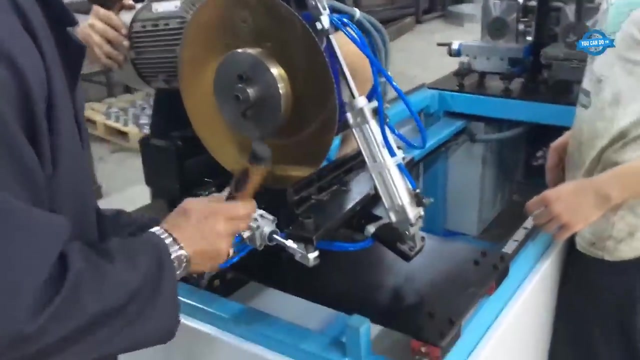 the machine to produce the desired flange. The machine also comes with a variety of safety features that help to prevent accidents and injuries. The Maket 20-30 flange machine is a high quality machine that is highly customizable. It can be configured to produce a wide range of flange sizes and shapes. 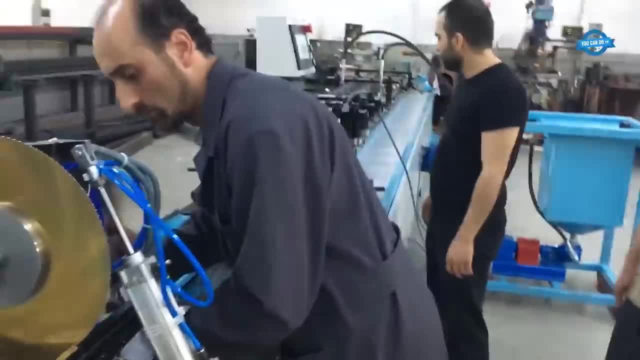 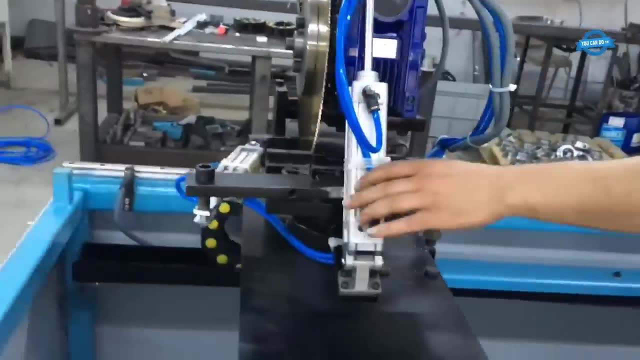 This means that it can be used to produce flanges for a variety of different applications. Another key feature of the Maket 20-30 flange machine is its energy efficiency. The machine is designed to use minimal energy, which means that it is both environmentally. 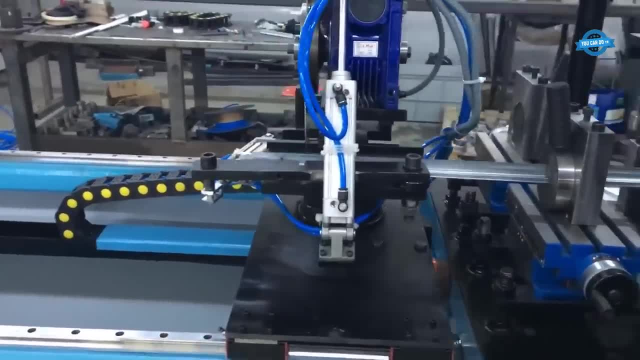 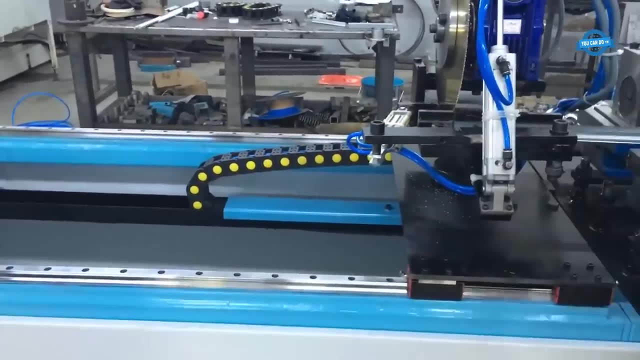 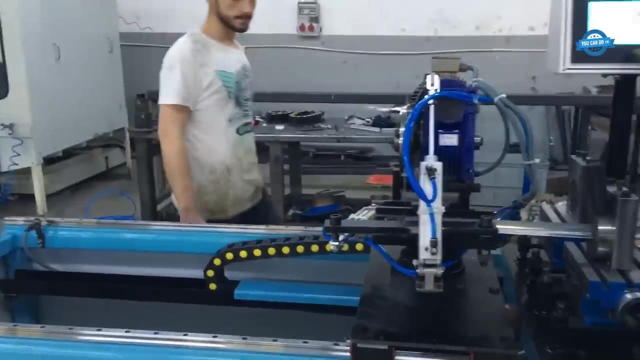 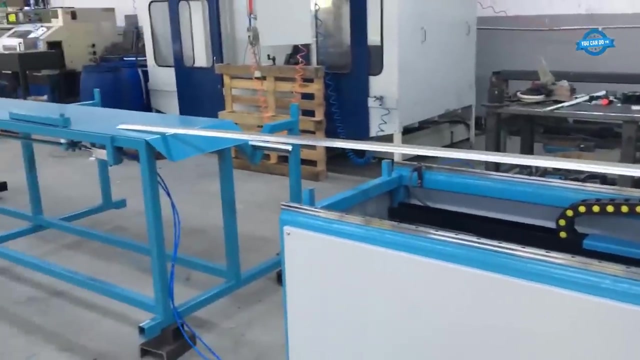 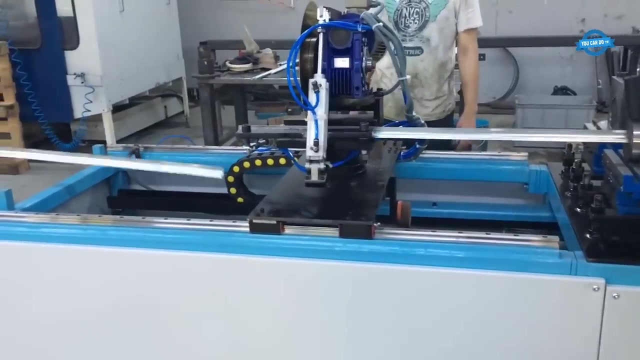 friendly and cost effective to operate it, an ideal choice for companies that are looking to reduce their energy costs and their carbon footprint. In addition to the Mackett 20 to 30 flange machine, Mackett also produces a range of other profile drawing machines. These include roll formers, which are used to create a variety 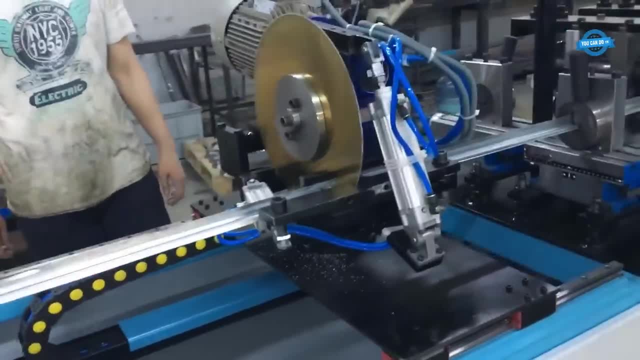 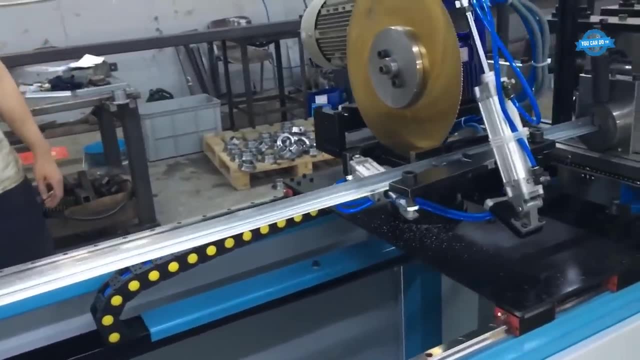 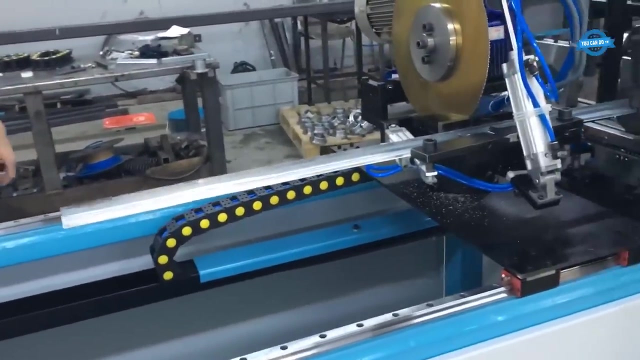 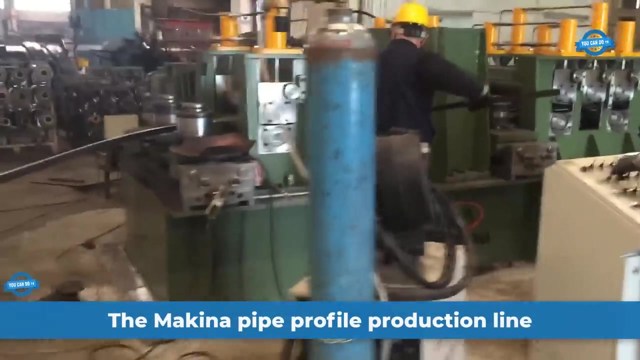 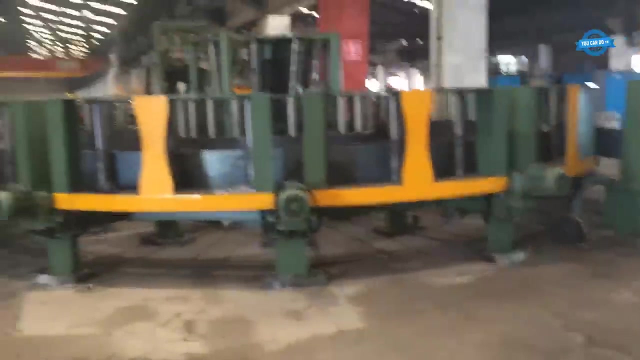 of different metal profiles and other flange machines that are designed to produce different types of flanges. The Machina Pipe Profile production line is an advanced manufacturing machinery designed to produce high quality and consistent pipe profiles in various sizes and thicknesses. The production line comprises: 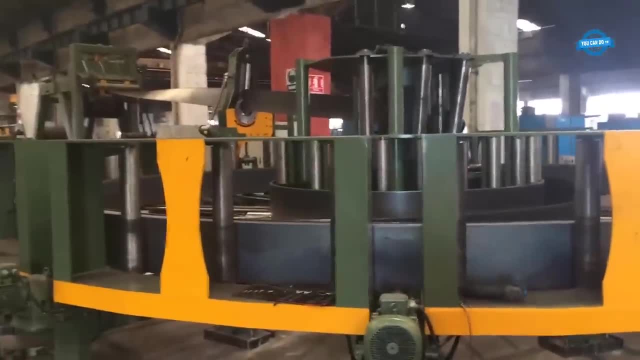 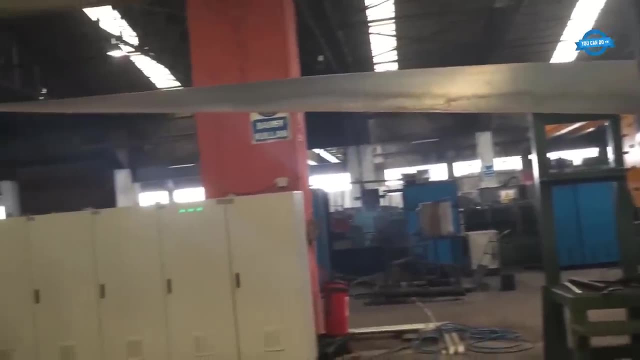 several machines and equipment, each with a specific function that contributes to the final product's creation. The first machine in the production line is the coil holder, which holds the steel coil. The coil holder feeds the coil to the uncoiler, which unwinds. 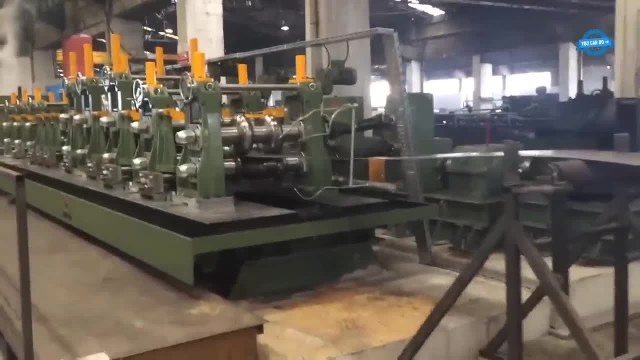 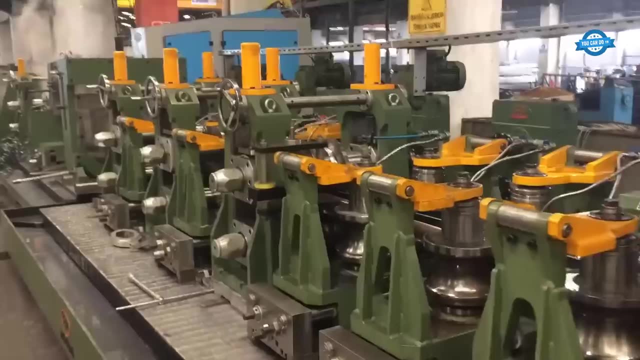 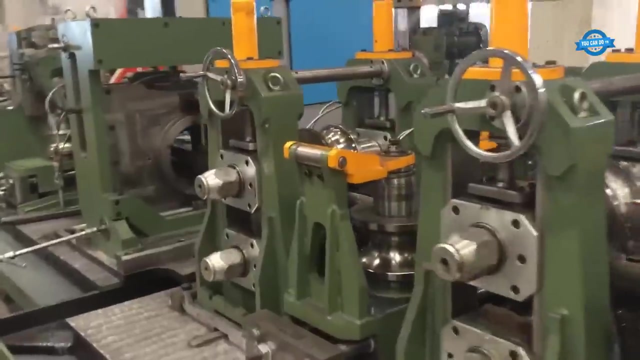 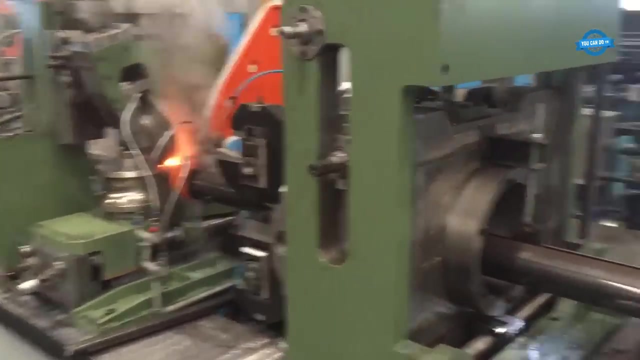 the steel coil and feeds it to the straightening machine. The straightening machine works by passing the steel coil through a series of rollers that exert pressure on the metal, straightening any kinks or bends. After the steel coil is straightened, the next machine in the production line is a roller. 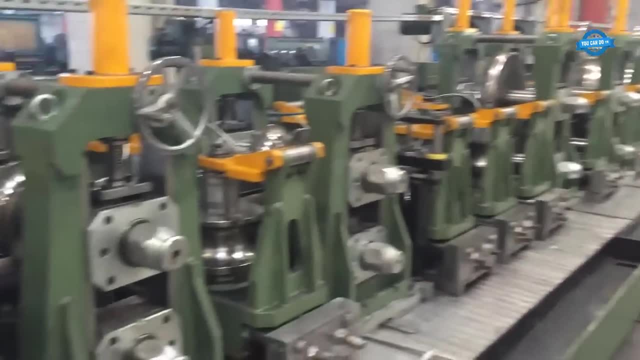 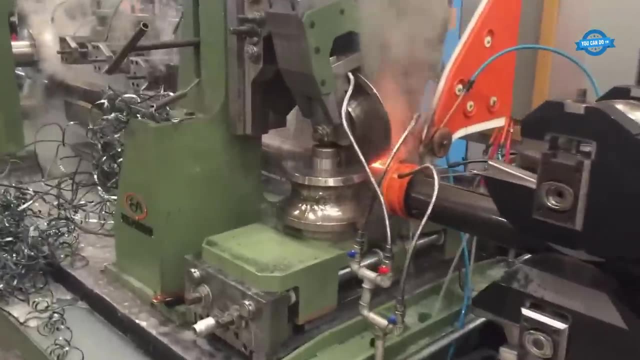 system that gradually shapes the steel coil into a round shape. The machine then carefully Finally a tubular shape. The roller system comprises a series of rollers that gradually bend the steel coil into the desired shape. This process is controlled and monitored by computerized systems that ensure the tube's 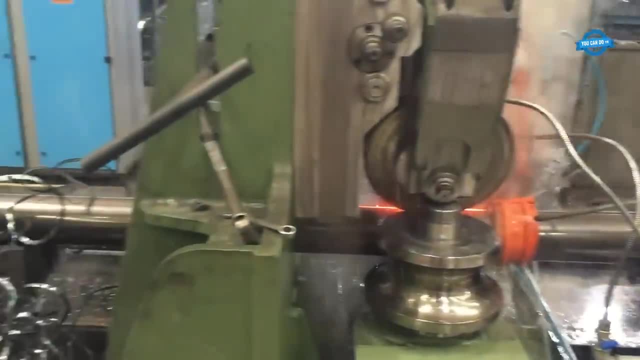 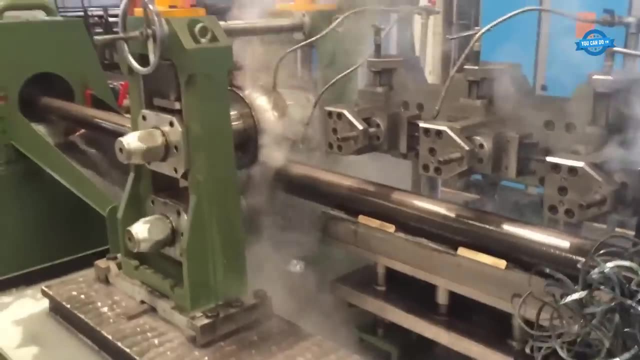 dimensions and shape are precise. Once the steel coil is formed into a tubular shape, the welding machine joins the two edges of the pipe to form a complete round pipe. The welding process uses high-frequency electric currents to heat and melt the metal edges. 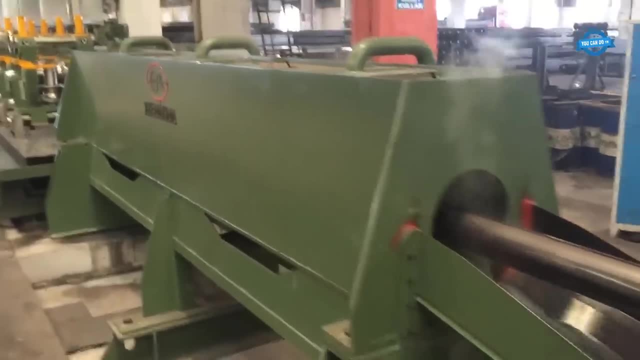 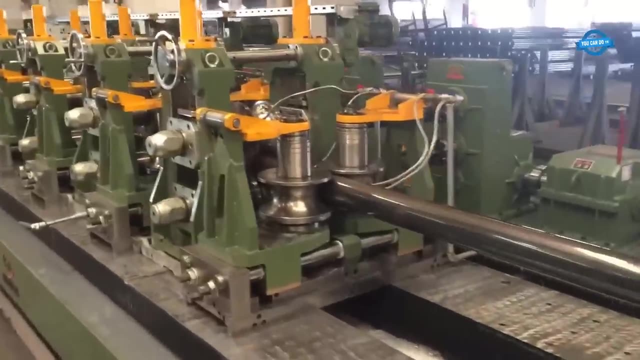 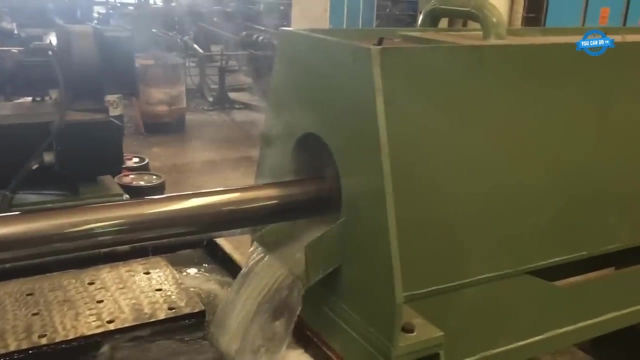 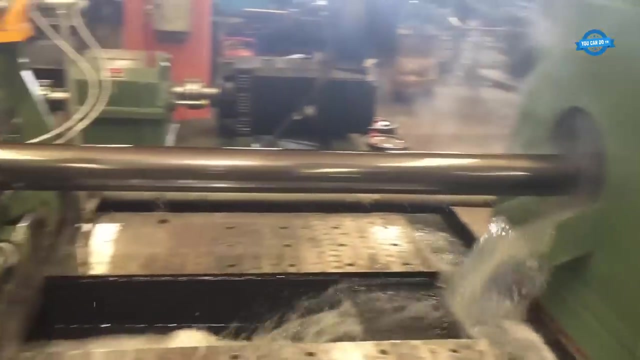 forming a strong and durable weld. After the welding process, the round tube continues to run through another machine that helps shape it into a rectangular or square box, depending on production needs. This machine is capable of shaping the tube in various sizes and dimensions, depending. 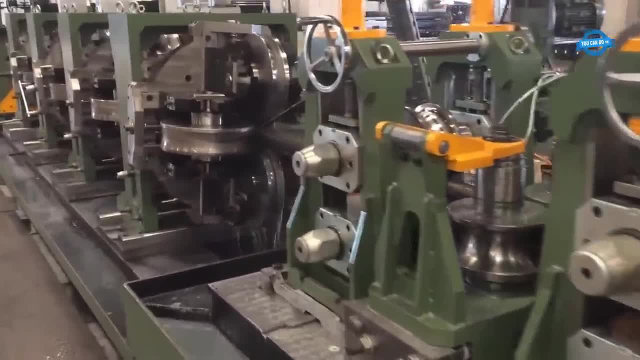 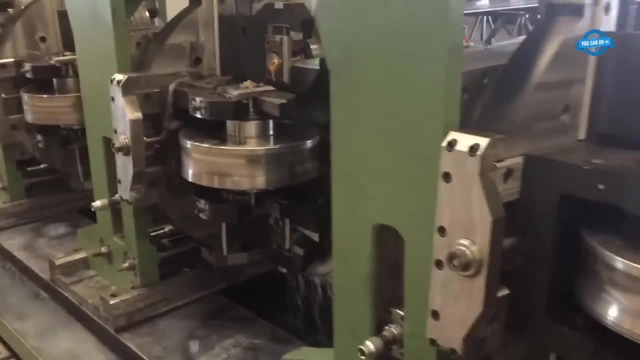 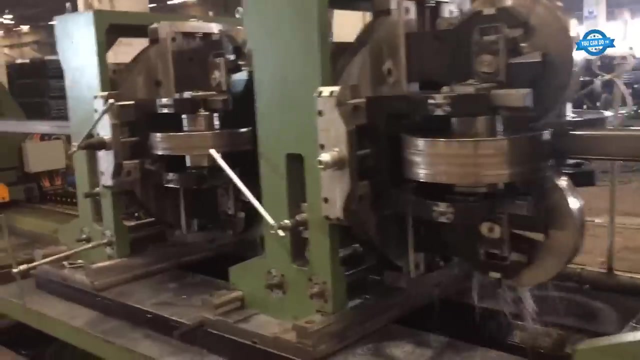 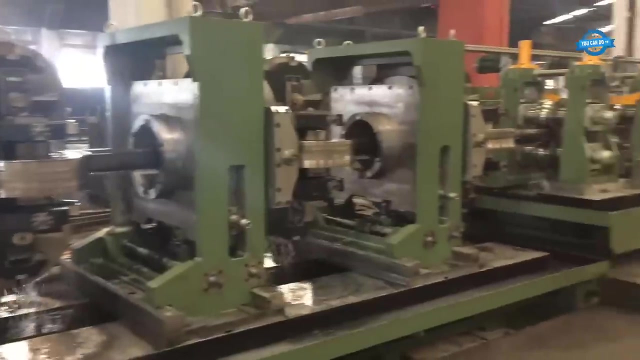 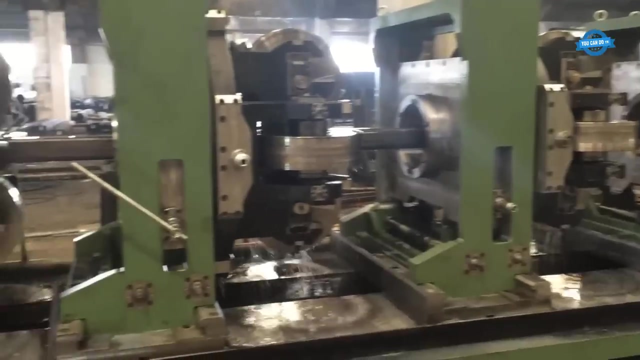 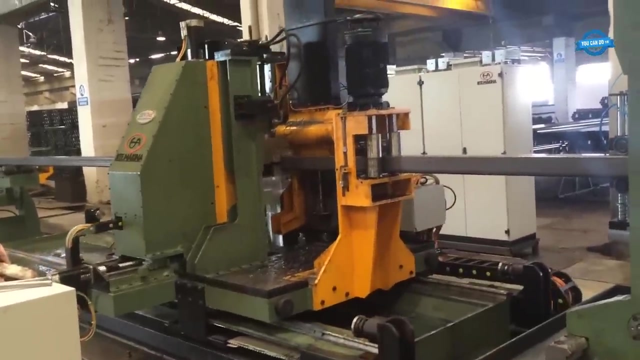 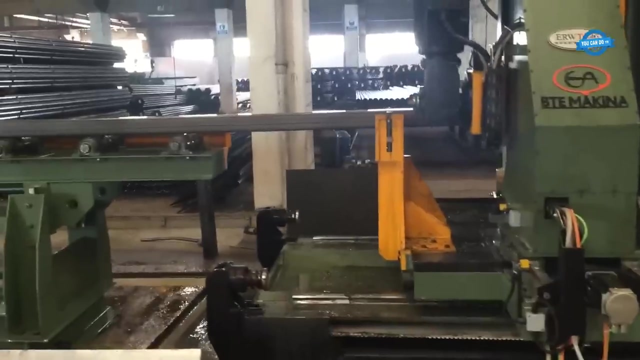 on the client's specifications. This machine is capable of shaping the tube in various sizes and dimensions, depending on production needs. The production line also includes a cutting machine that cuts the pipe to the desired length. This machine is programmed to cut the pipe accurately and efficiently, ensuring minimum 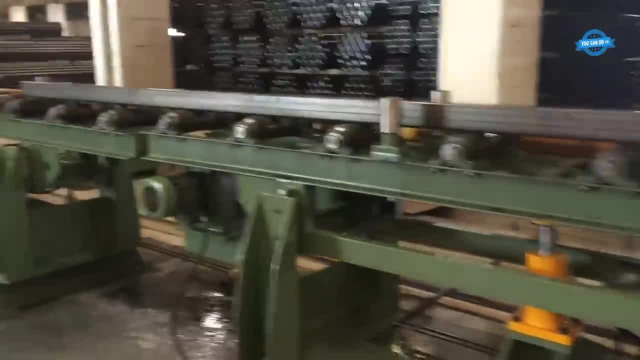 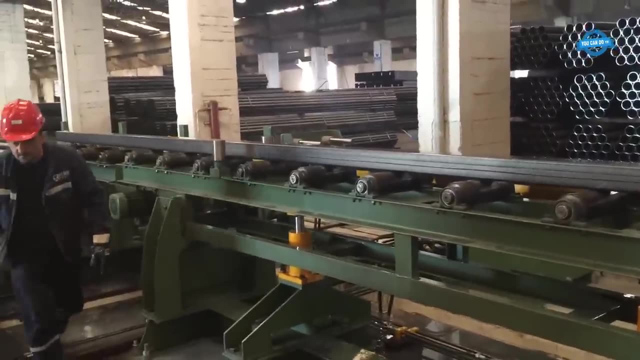 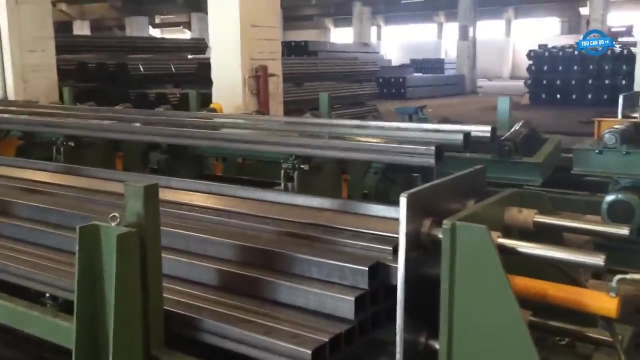 waste and maximum productivity. The Machina pipe profile production line is suitable for producing a wide range of pipe profiles, including square, rectangular and circular profiles. The machine can produce pipes in various sizes and thicknesses, ranging from 10mm to 219mm. 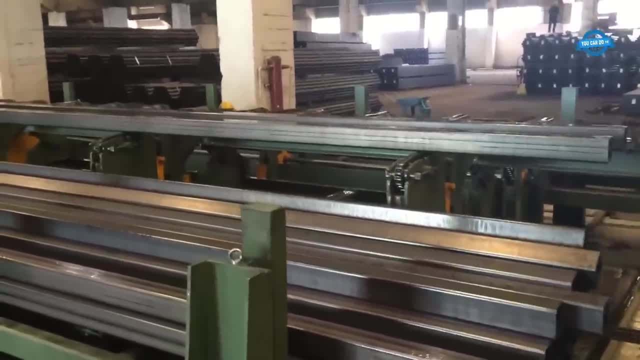 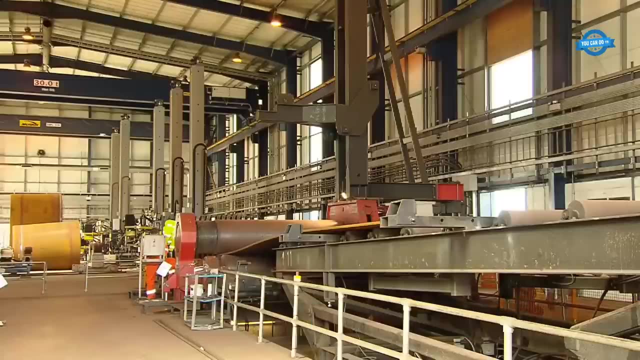 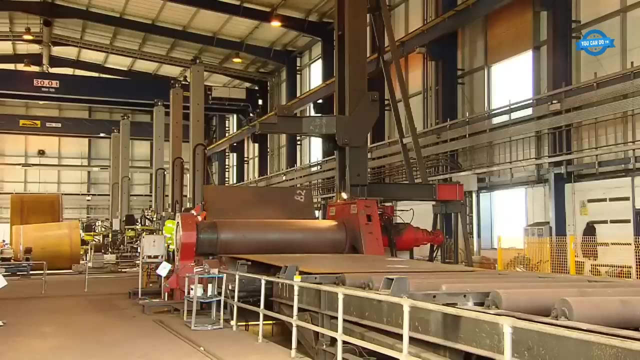 in diameter and up to 10mm thick. This short video showing the process of manufacturing a wind tower at Wind Tower Scotland Limited in Campbelltown, Scotland's only wind tower manufacturing facility. The raw material is large, flexible and easy to use: Flat sheets of steel that will form the cylindrical sections of the wind tower. 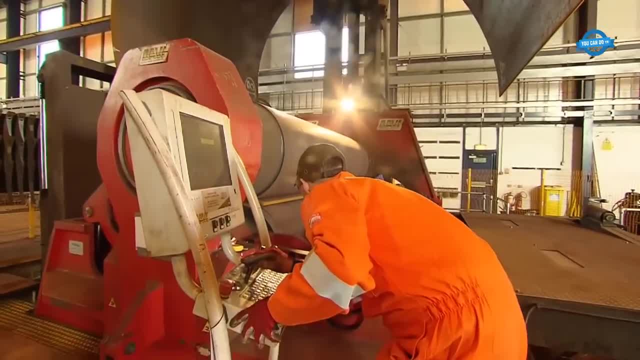 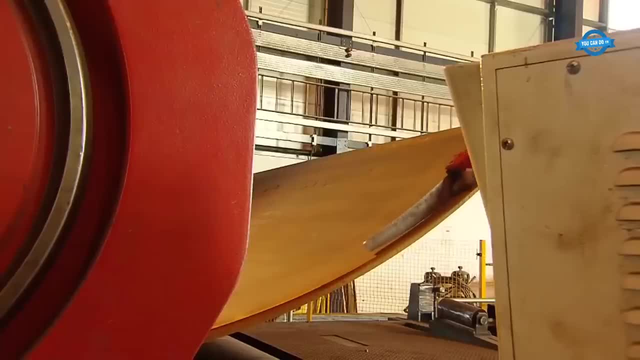 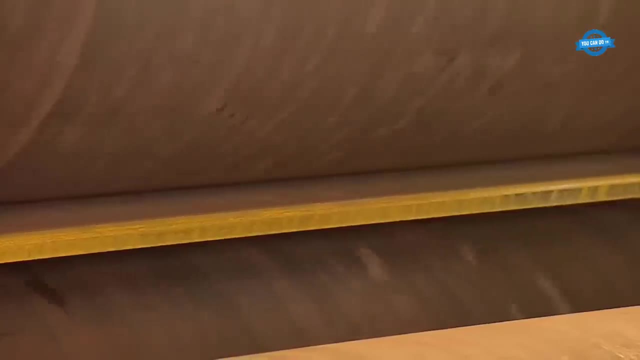 The plate rolling machine is used to bend the steel plates into the desired shape. This machine consists of four rollers. The machine is set up by adjusting the position and gap between the rollers according to the required bending radius and plate thickness. A steel plate is carefully inserted into the machine, ensuring it aligns properly with 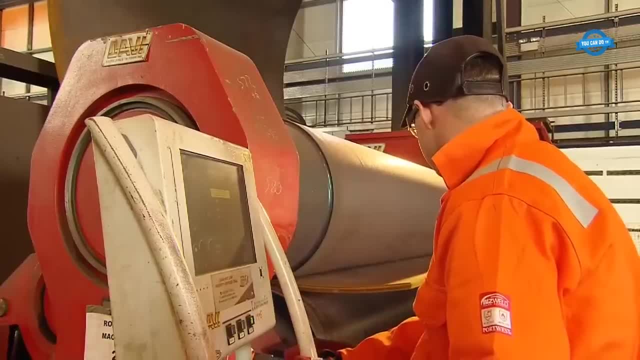 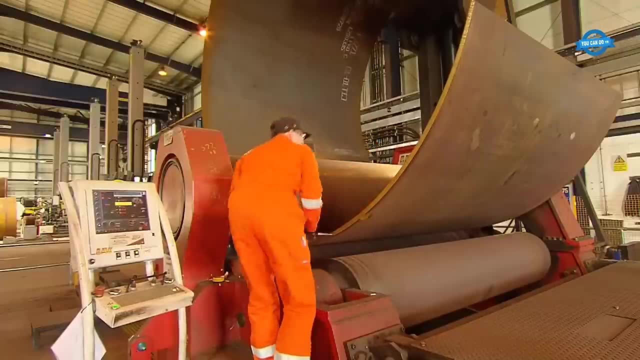 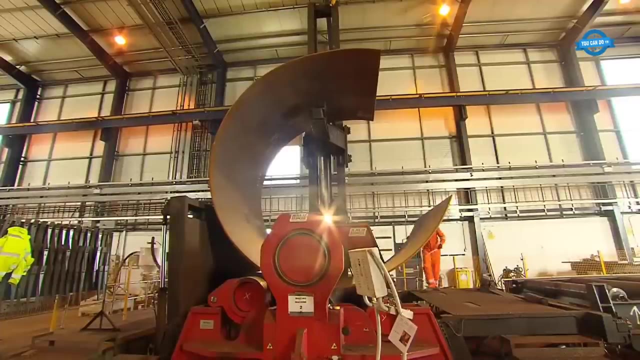 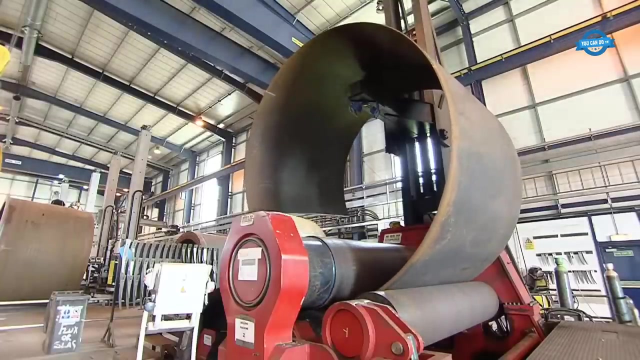 the rollers. The machine's hydraulic system exerts pressure on the plate, gradually bending it around the rollers. The plate is passed through the machine multiple times to achieve the desired curvature. Depending on the wind tower's design, several steel plates may be bent using the roller. 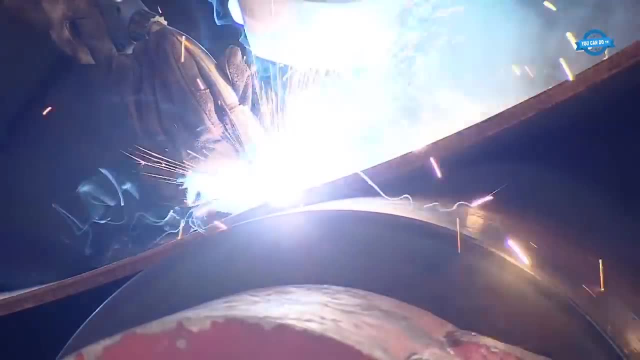 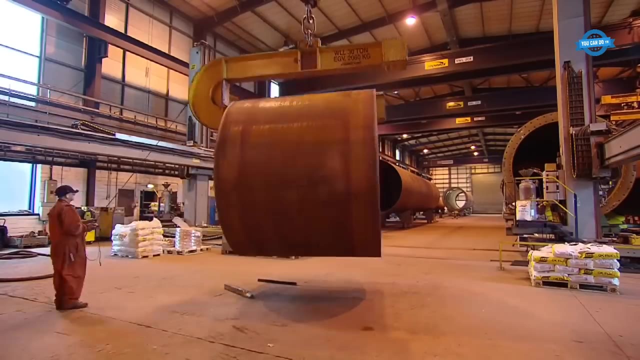 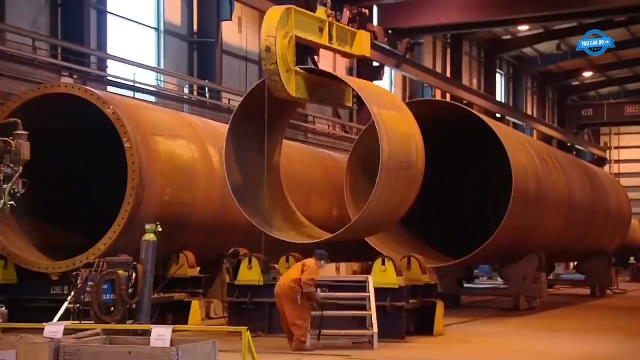 bending machine to form different sections of the tower. Throughout the bending process, quality control checks are conducted to ensure the accuracy and precision of the bends. Measurements are taken to verify that the bending radius and angle meet the specified requirements. Once the steel plates are bent into the desired shape, they are welded together to form the